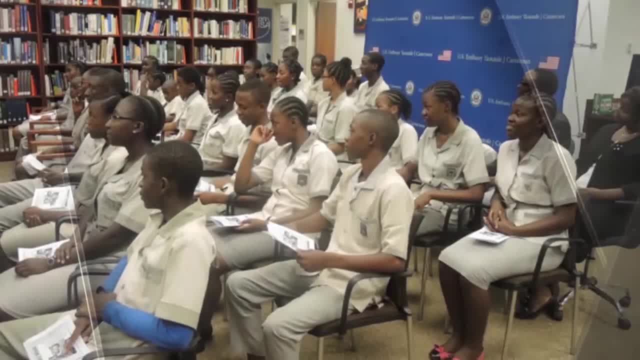 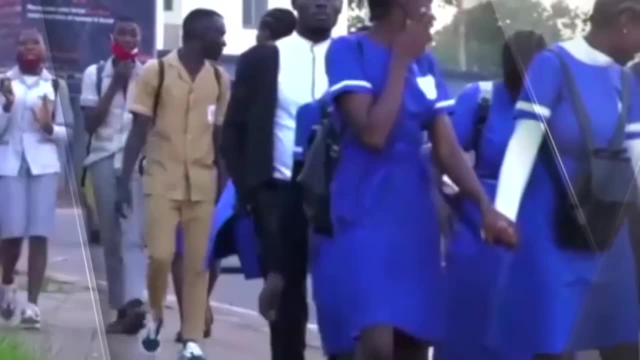 distance learning as another teaching and learning method which is different from the traditional classroom setting that you are all used to. In the distance education mode, you are not with the teacher in person, so take your time, relax, listen to the teacher. 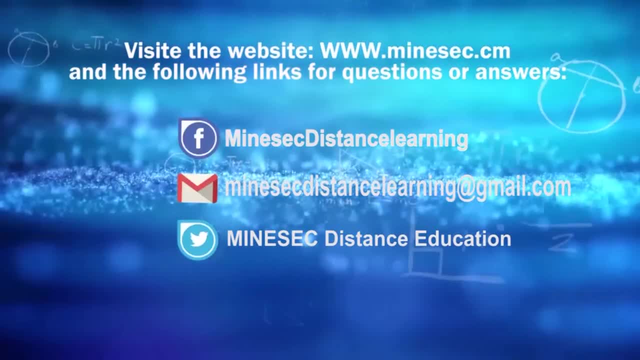 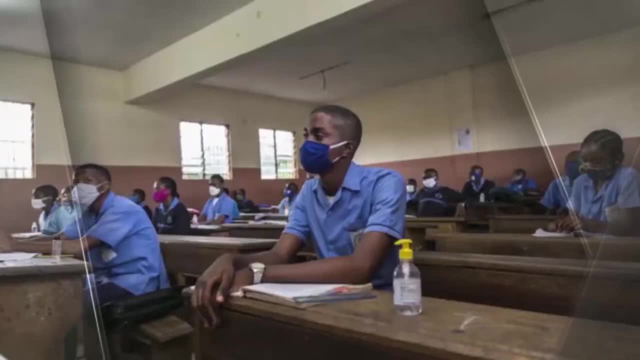 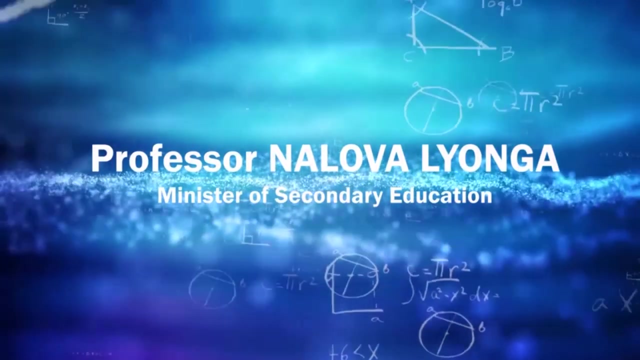 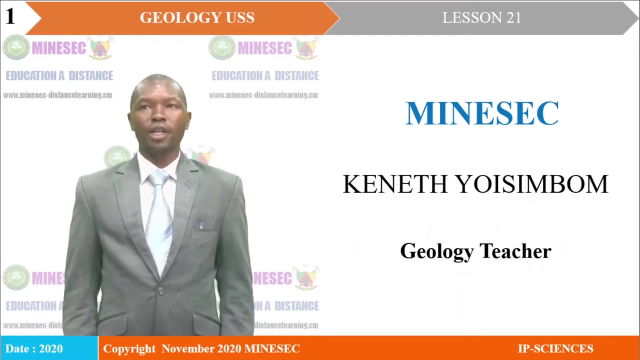 take down notes and visit the following links for any questions or answers to your questions. Take it in your stride. This is Cameroon's solution to COVID-19 and beyond. Professor Nalovalyonga, Minister of Secondary Education, Welcome to lesson 21 of your distance learning program for Geology. Opposite Science with 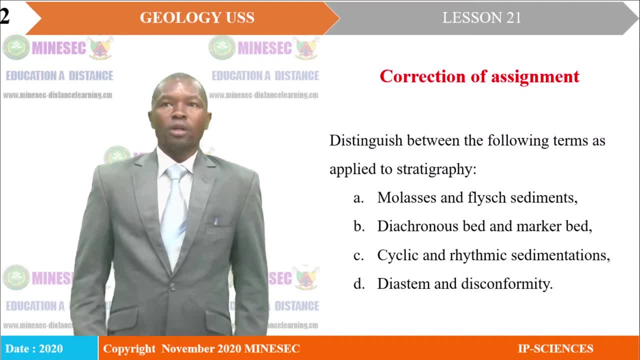 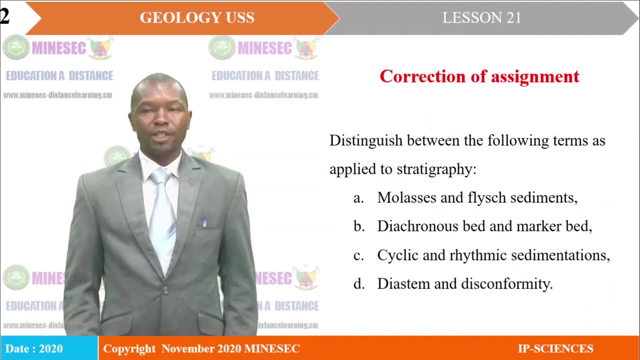 Kenneth Yosimbong During our lesson 21,. we had an assignment. We shall proceed by correcting the assignment. The assignment required that, firstly, you distinguish between the following terms, as applied to stratigraphy: A path monox and flashy sediments or molasses. 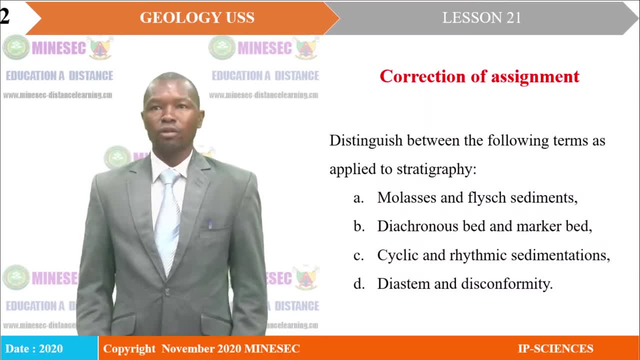 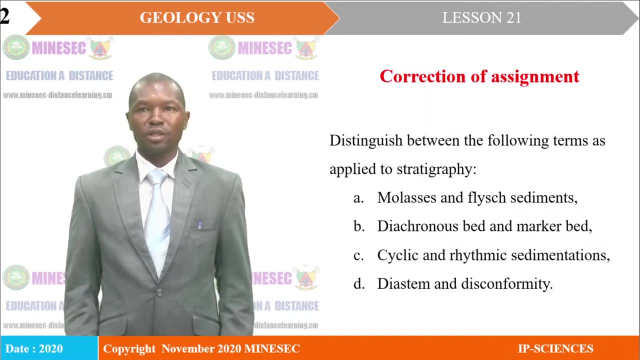 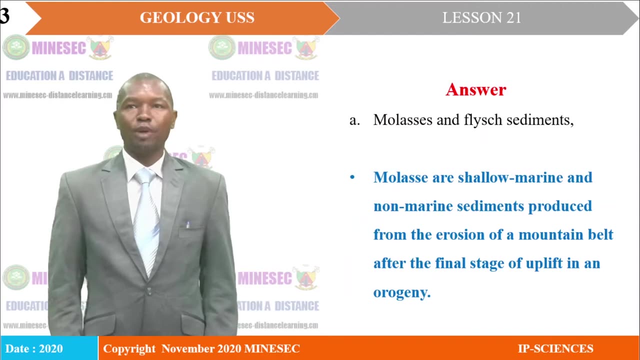 B- diachronous bed and marker bed. C- cyclic and rhythmic sedimentations. D- diasterect and disconformity. Now the first part of the question, which required that we should distinguish between molasses and flashy sediments. 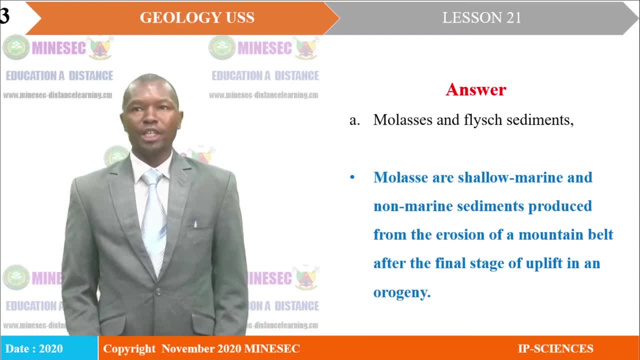 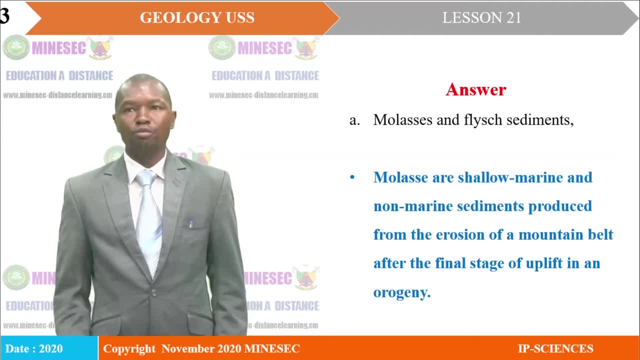 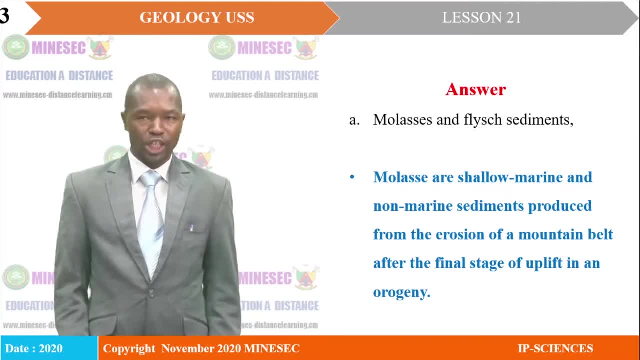 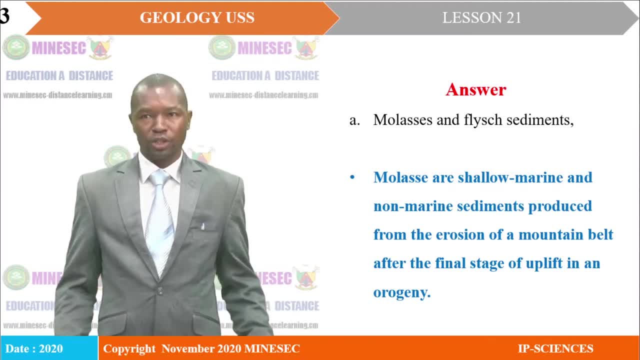 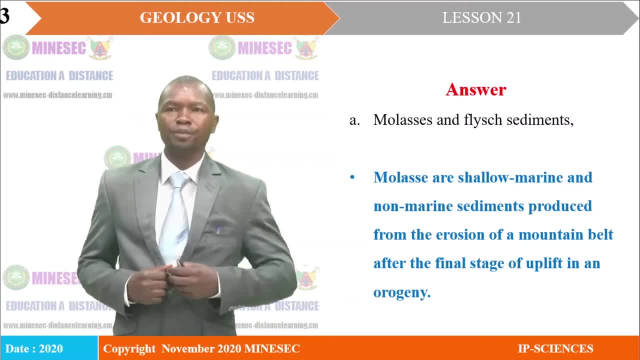 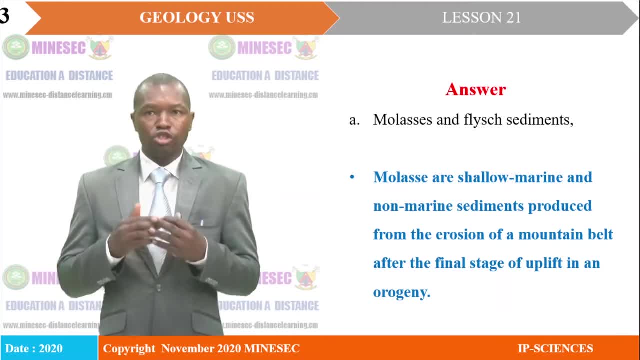 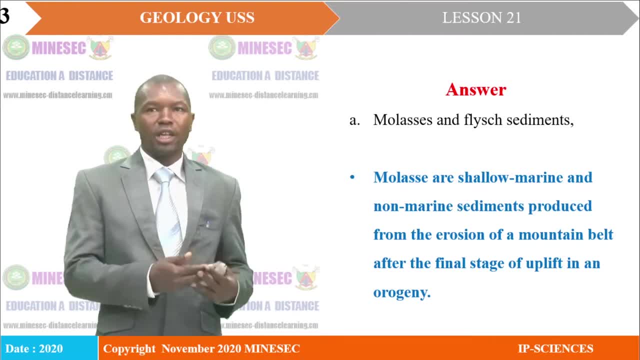 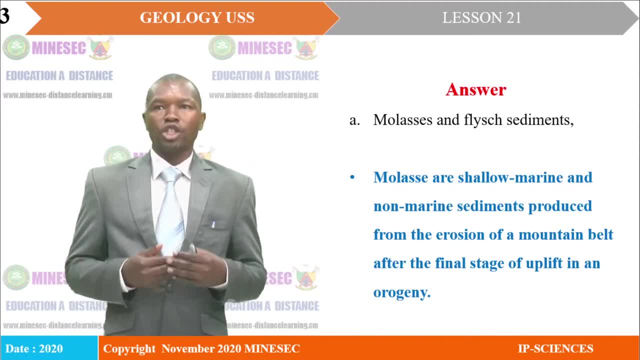 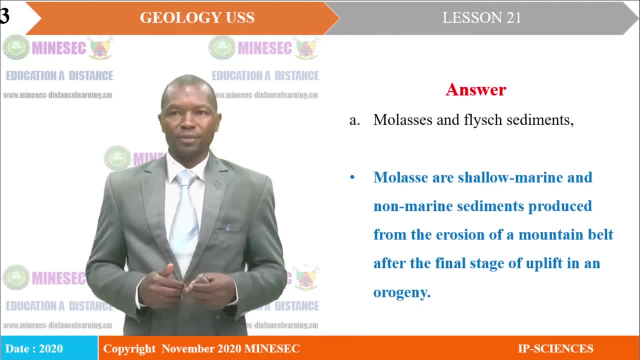 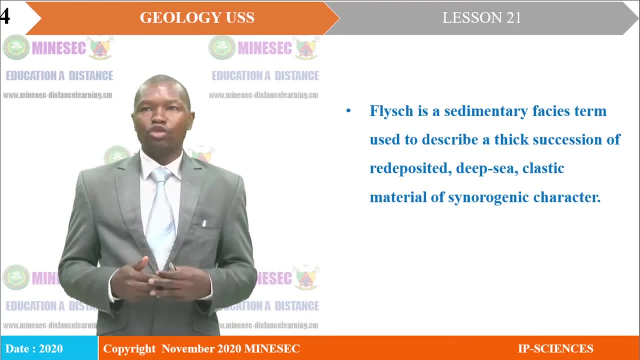 Molasses are shallow marine and non-molasses. Molasses are shallow marine and non-molasses is a sedimentary fashy term used to describe a thick cessation of redeposited gypsy clastic material of synerogenic character. 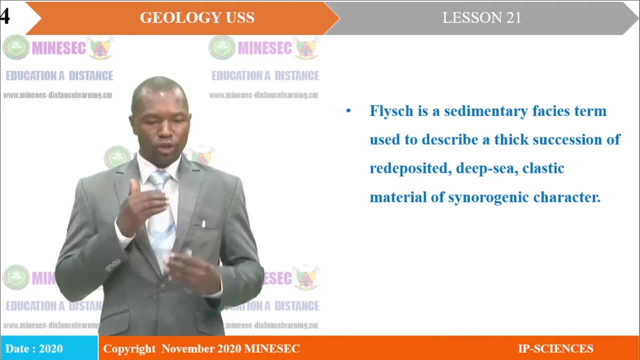 Remember that it's clastic, which means that it's material that has suffered weathering, erosion, transportation, being deposited before and preserved before they are being transformed to sedimentary rocks that now make the fashies, And remember that they are deep sea materials. 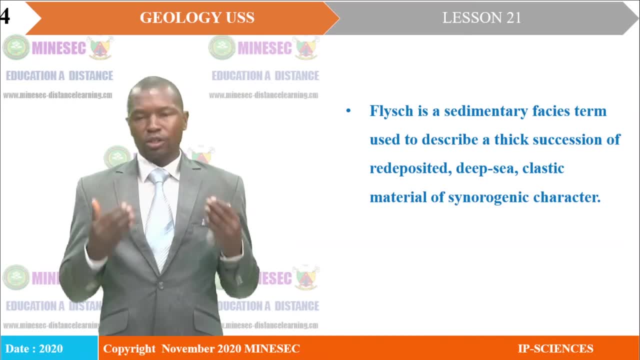 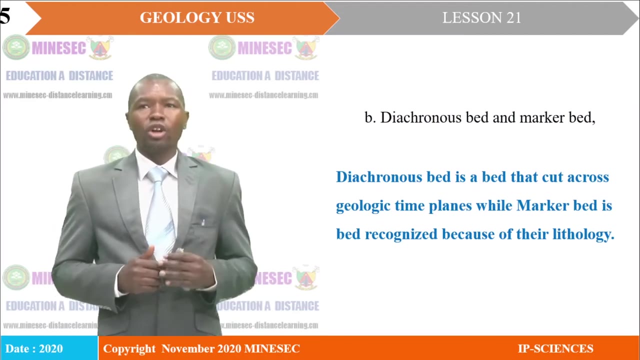 And deep sea. here should be environments where conditions are quiet and the degree of deoxygenation is also at the right. Dichronous bed and maca bed. Dichronous bed is a bed, A bed that cuts across geologic time planes. 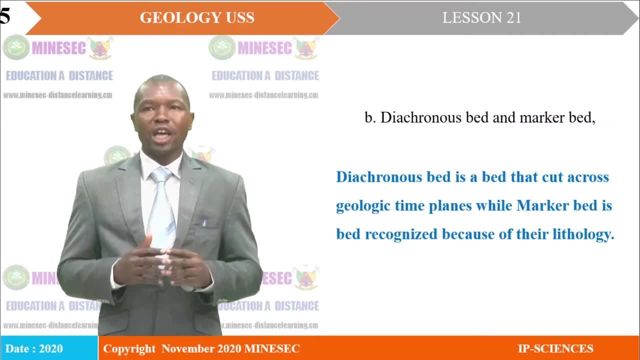 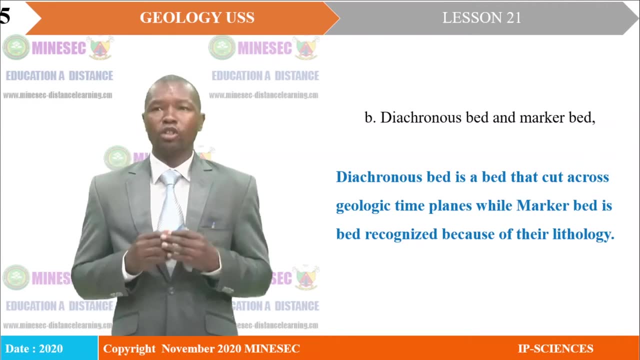 While a maca bed is that bed that is recognized because of its lithology, Or maca bed will be beds that are recognized because of their lithology. Therefore, the thin line difference here is that of the fact that a dichronous bed 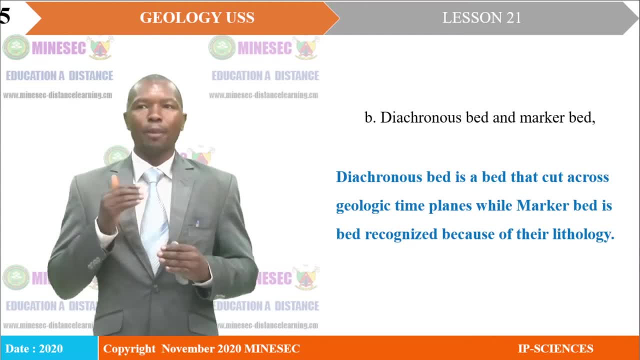 will cut across a geologic time plane, While a maca bed will simply be A maca bed will be recognized based on lithology. So it is possible that a dichronous bed could be a maca bed. It is possible. 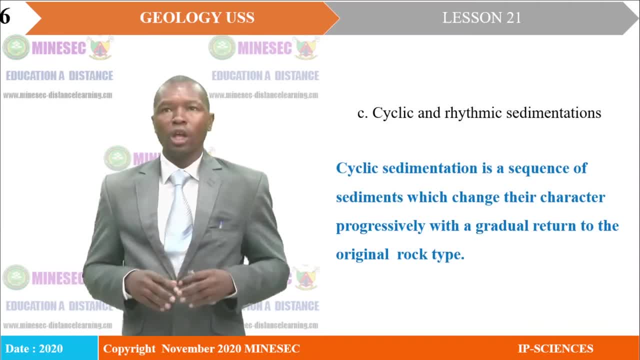 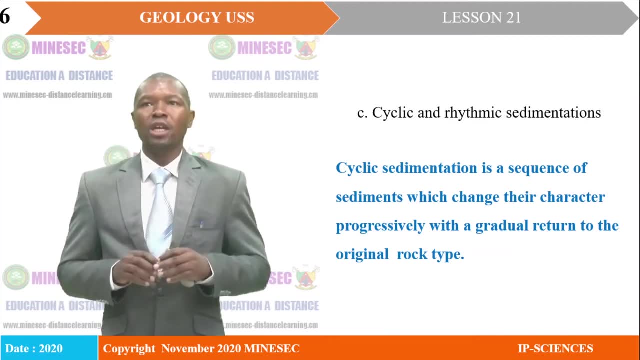 It may not be the same: Cyclic and rhythmic sedimentation. In cyclic sedimentation we underline the fact that here the sequence of sediments will change their character progressively, from one extreme to the other, with a gradual return, With a gradual return. 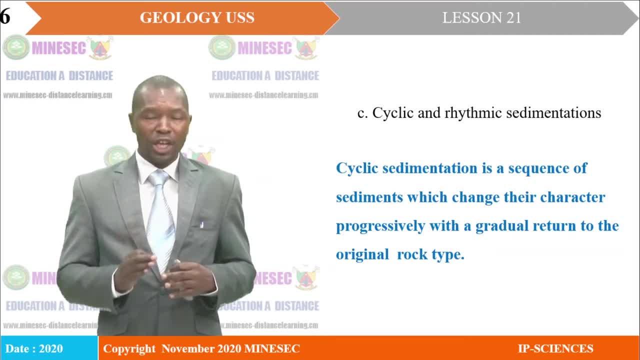 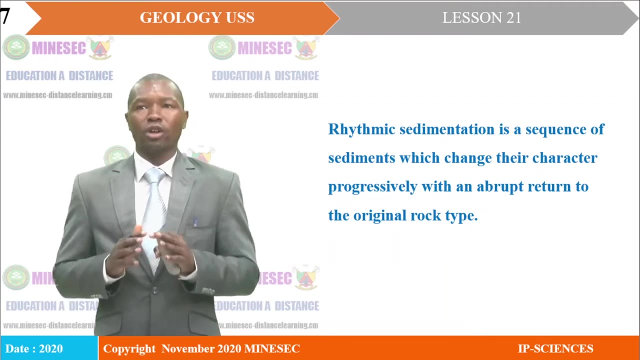 To the original rock type. Here the key word is the fact that there is gradual return to the original rock type, Whereas in rhythmic sedimentation there is an abrupt return to the original rock type, with the same sequence of sediments changing from one character, progressively from one extreme, to another. 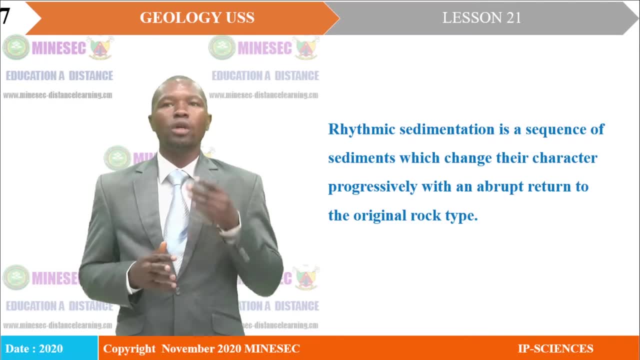 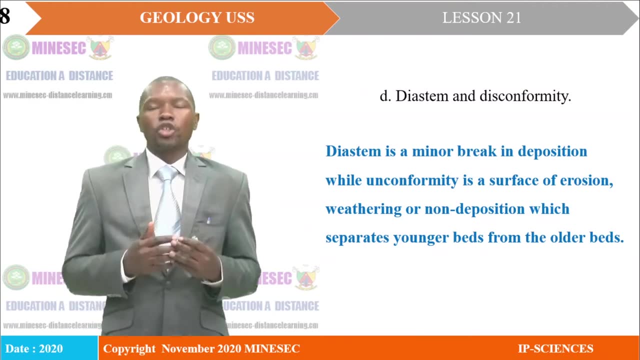 But with an abrupt return to the original rock type. But with an abrupt return to the original rock type, But with an abrupt return to the original rock type. Dijstem and disconformity: Dijstem is a minor break in deposition. 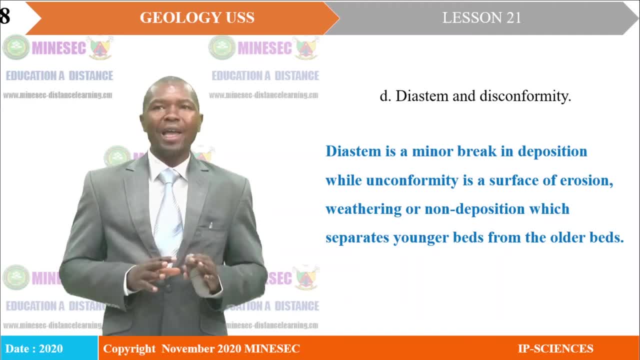 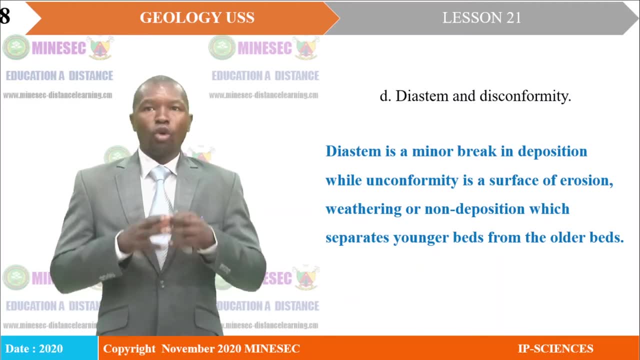 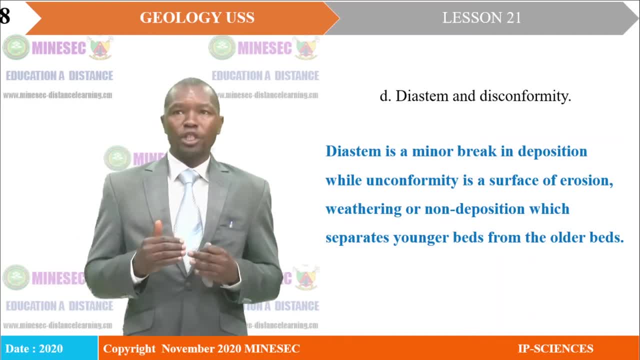 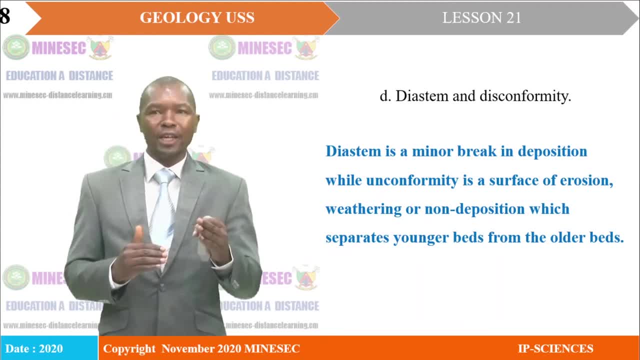 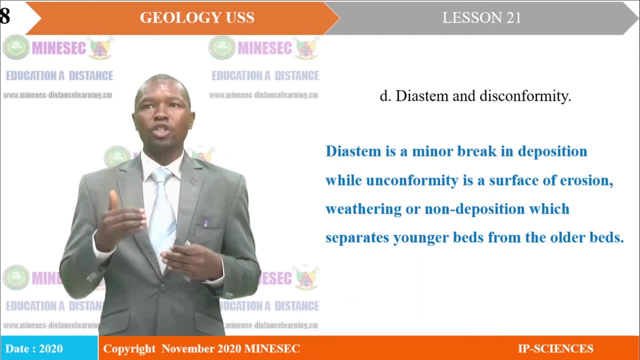 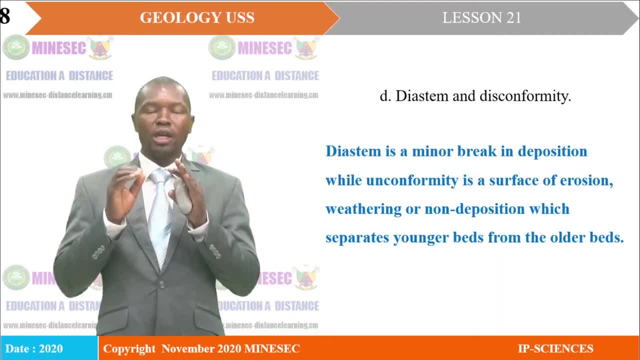 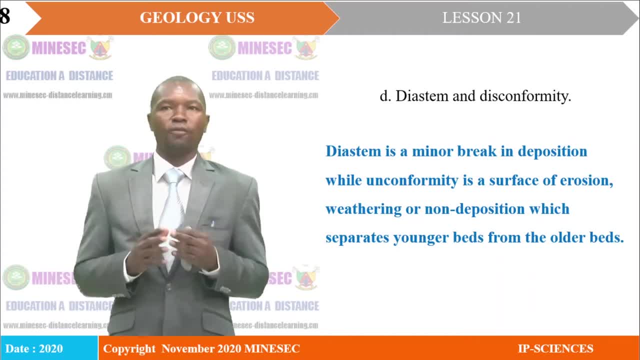 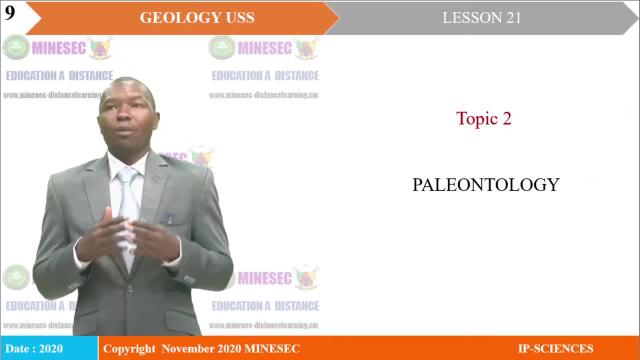 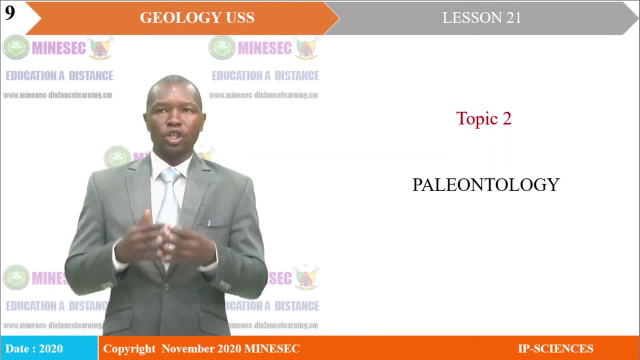 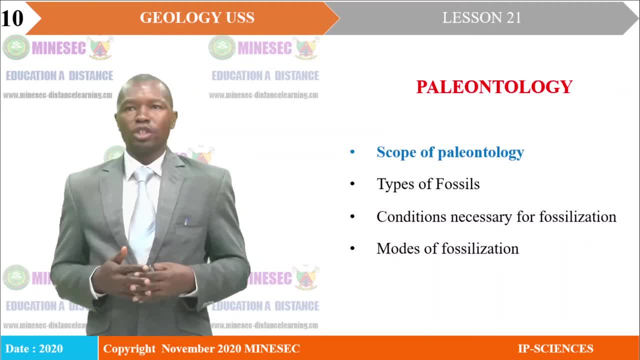 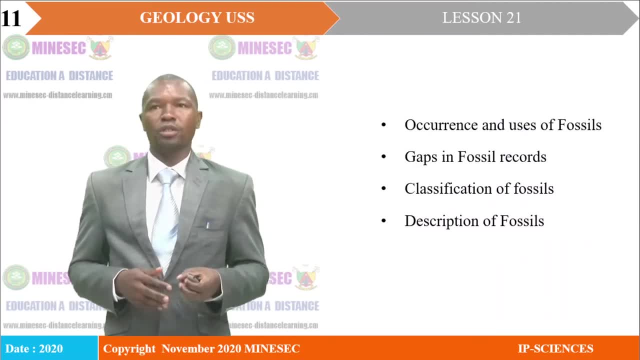 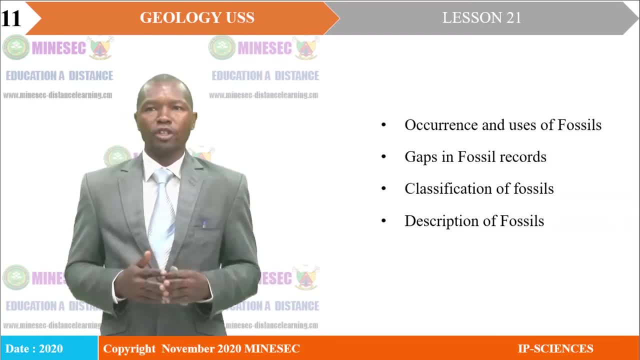 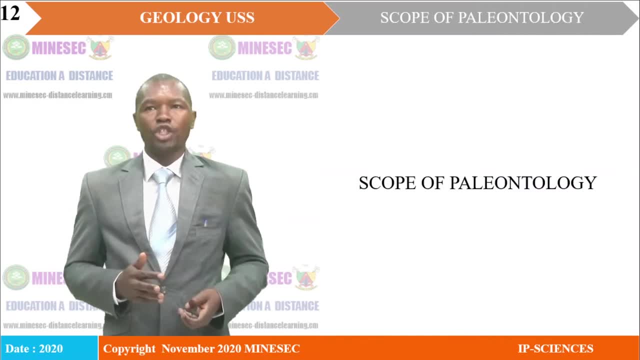 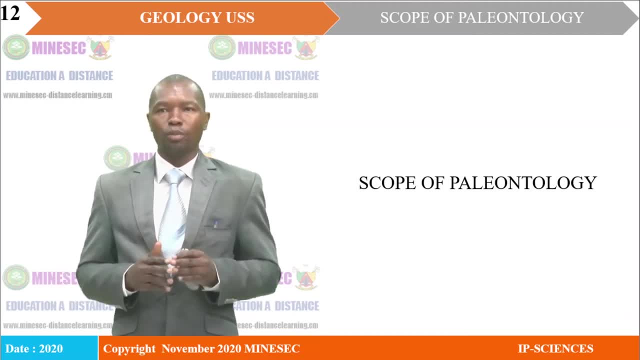 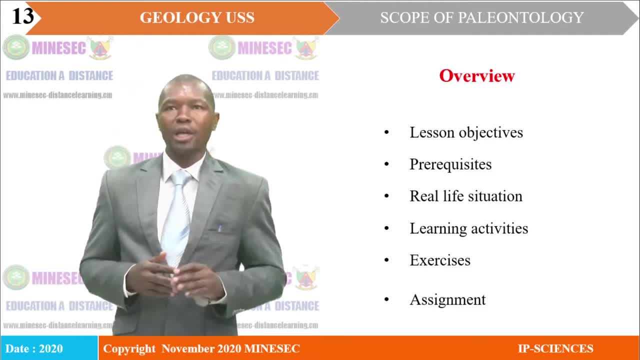 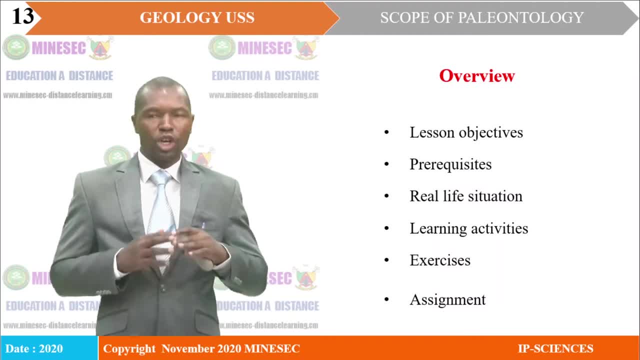 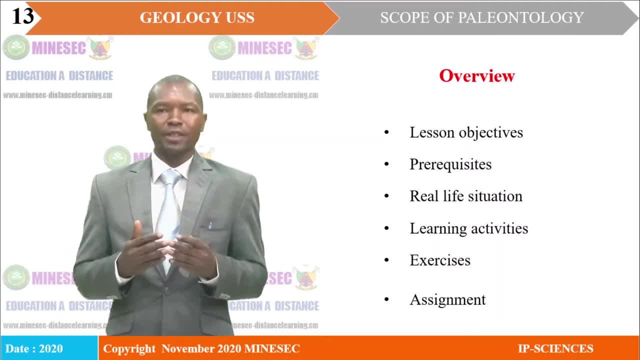 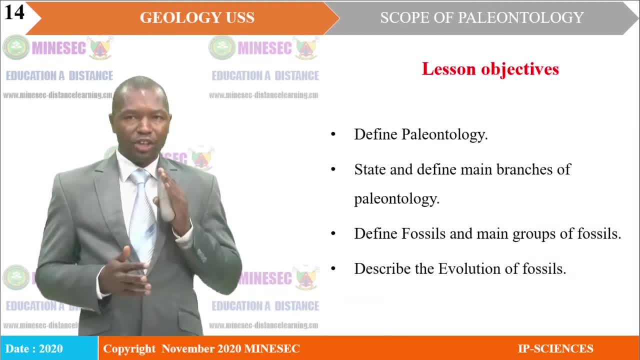 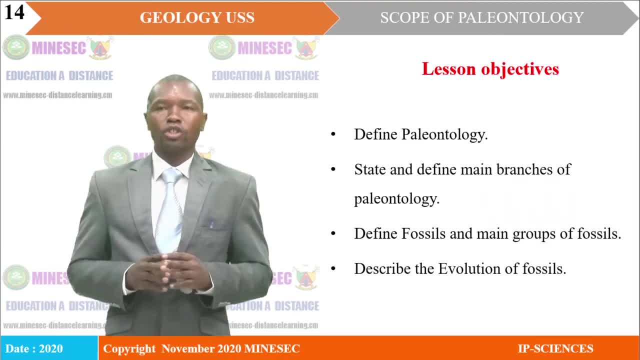 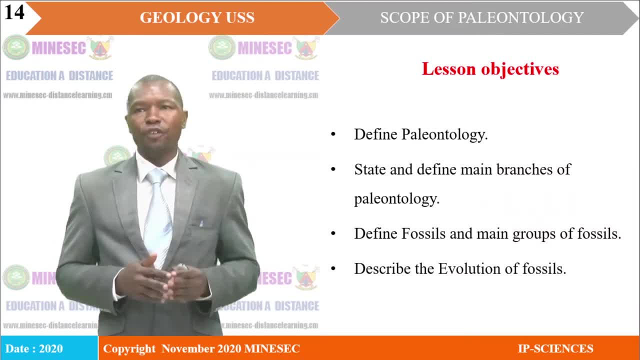 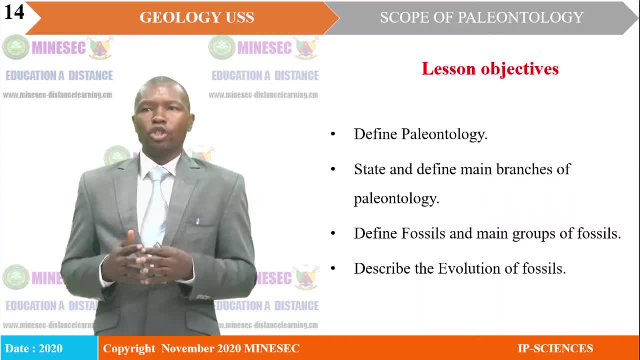 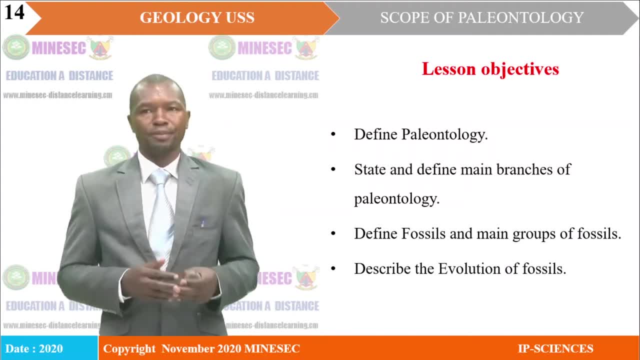 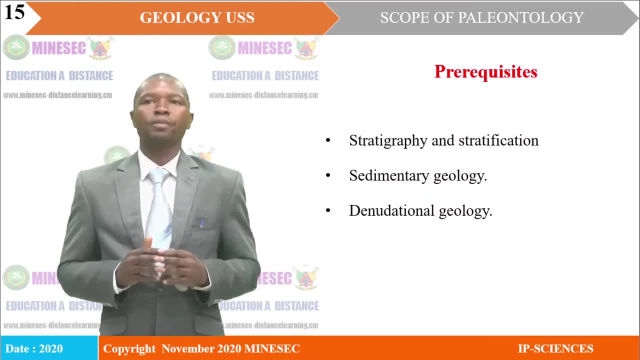 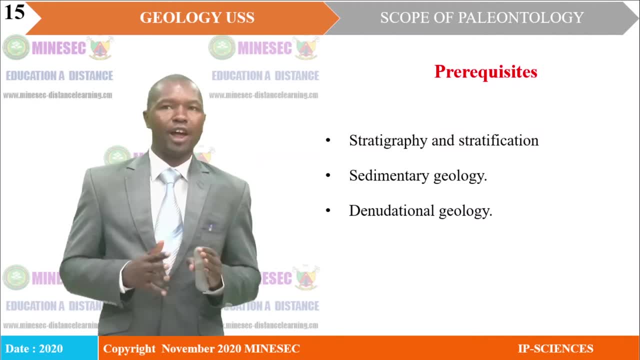 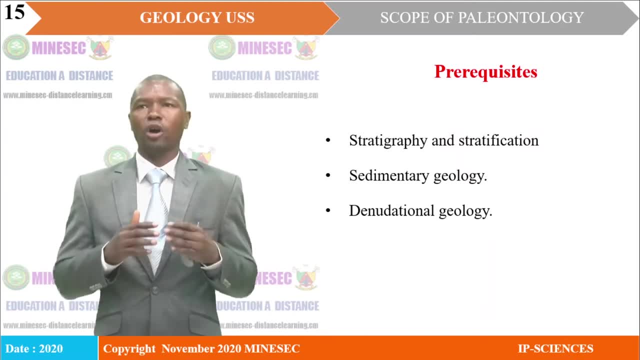 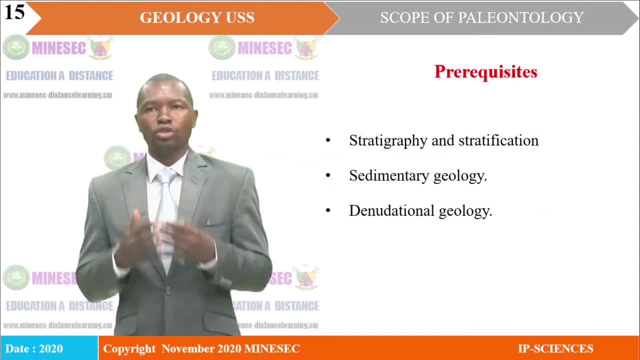 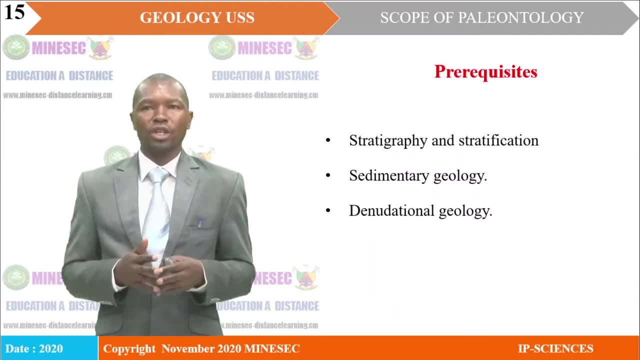 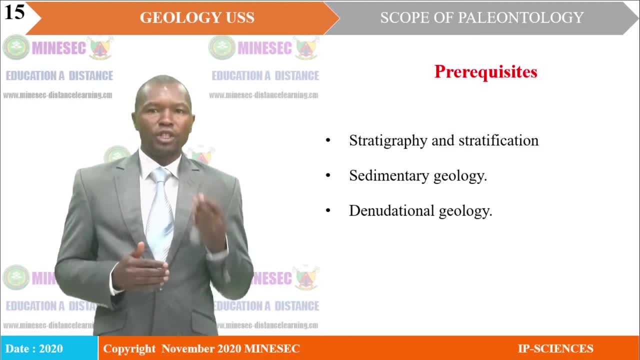 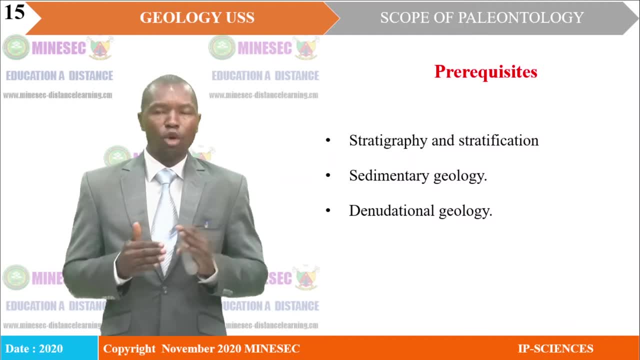 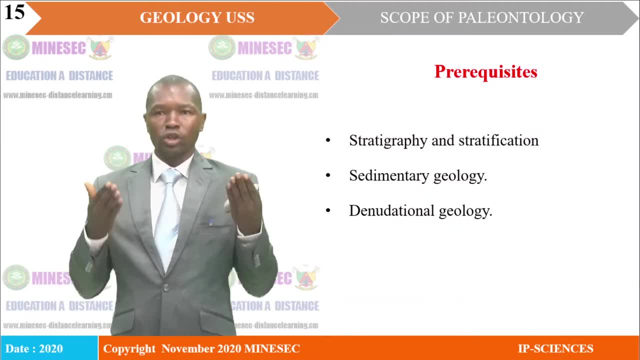 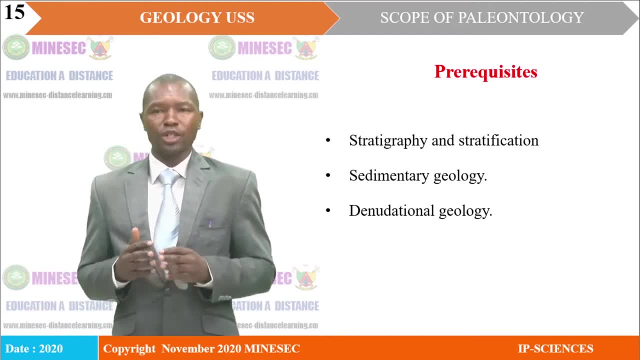 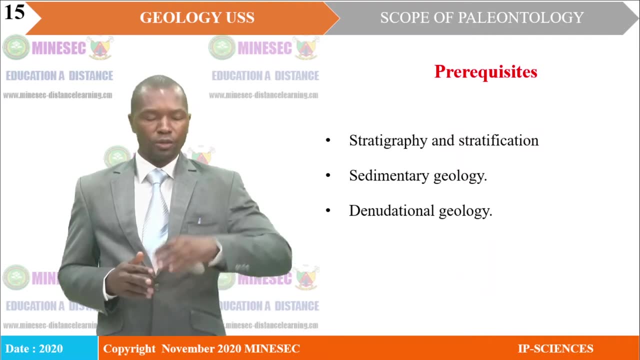 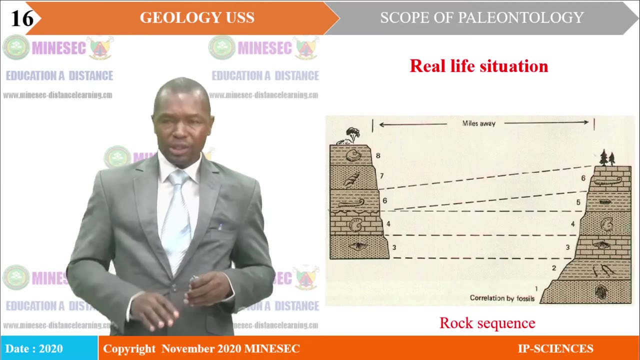 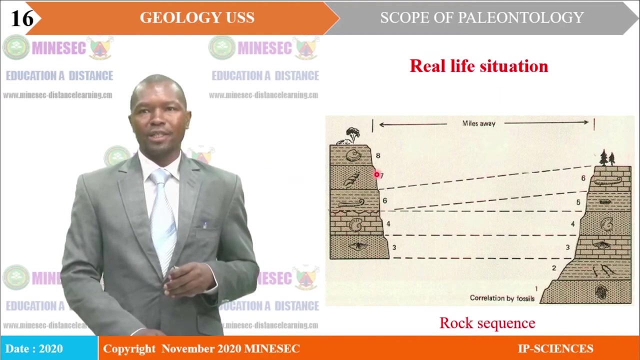 Which separates human body from the earth, Which separates human body from the earth. That brush cannot eat my breath anymore. That brush cannot drink my pee anymore. But yeah, We will keep laughing. Let's watch first particular fossil species. now a geologist observed this, possibly an engineering geology. 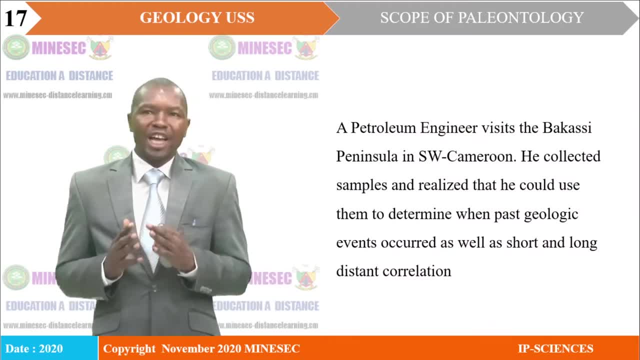 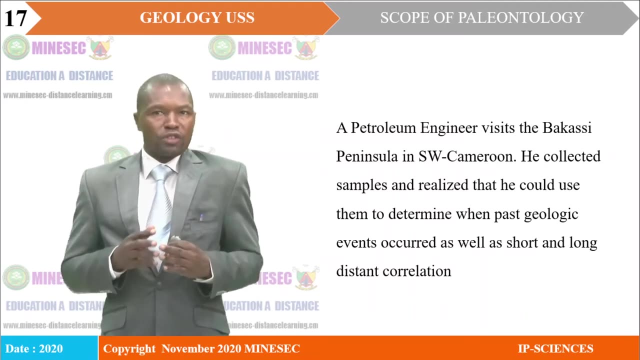 a petroleum engineer visits the bakashi peninsula in the southwest cameroon with the picture of the photo or the rock sequence we have. he collected samples and realized that he could use them to determine when past geologic events occurred, as well as short and long distant correlation. that is what he realized with the reflection of the photo we are just from seeing. 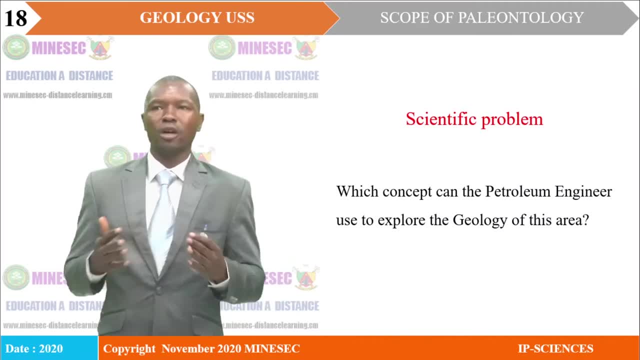 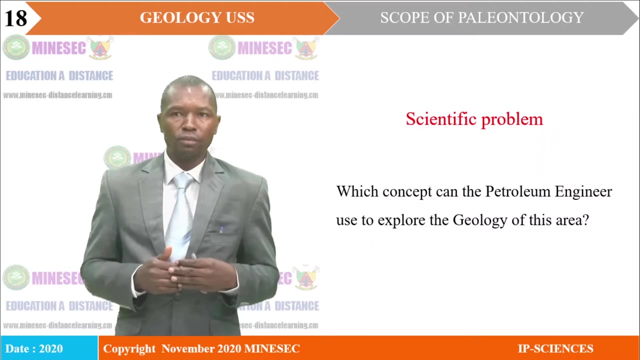 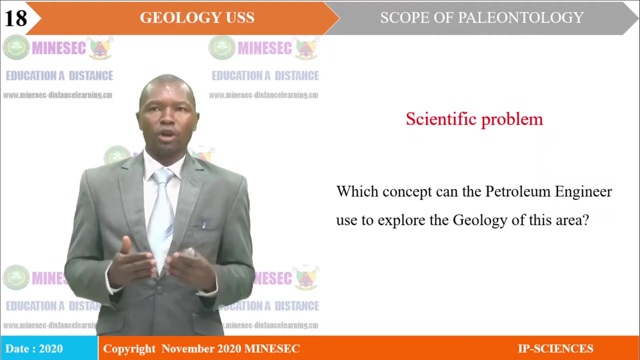 in his mind. now the scientific uh situation that we need to solve in this case will be: which concepts can the petroleum engineer use to explore the geology of this area? going to have some hypotheses which we presume should be able to help him resolve. the first hypothesis is supposed to use. 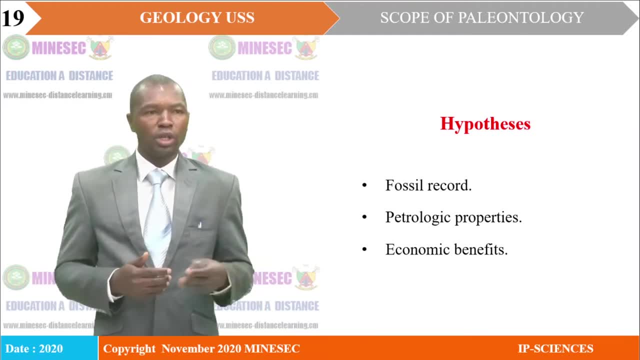 a fossil record because he realized that he could date information, some geologic information, in the past. maybe he could use the petrologic properties, since it also required that he should date the geology of the past. but that's still the economic benefits of the materials. these are our hypotheses as we 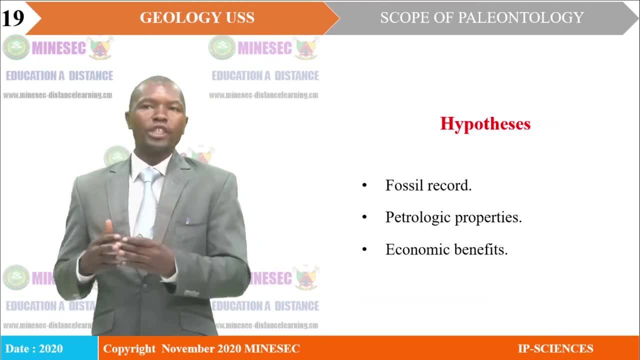 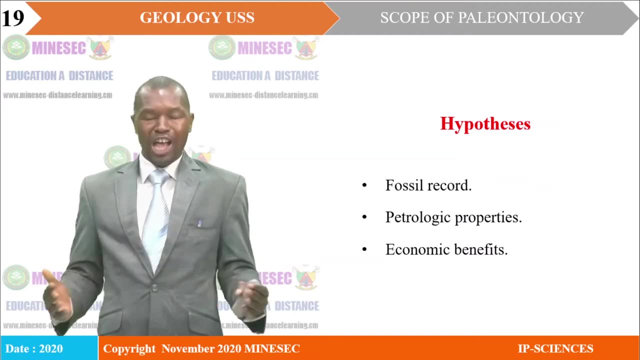 go through our lesson, we will be able to know which of the hypothesis will help the engine, the petroleum engineer, to be able to understand the geology of the past, as well as correlate rocks, and so then it will help us to be able to generally grasp the scope of geology, or the scope of 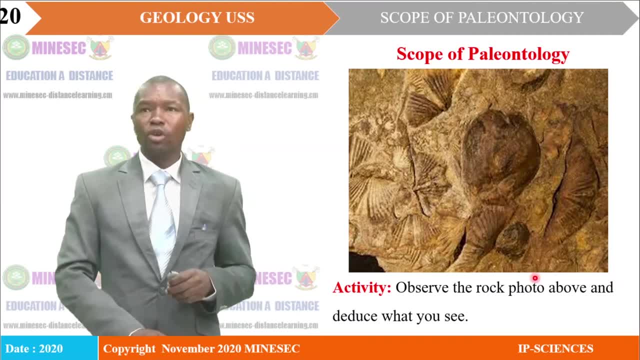 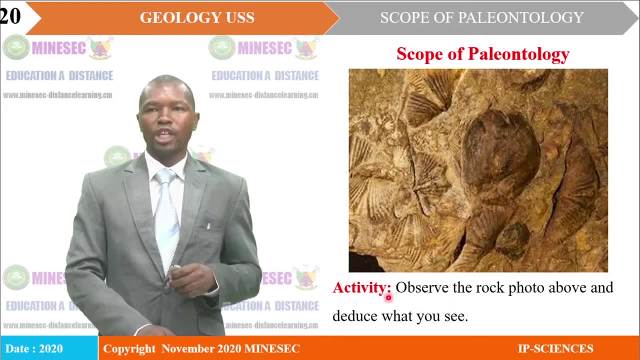 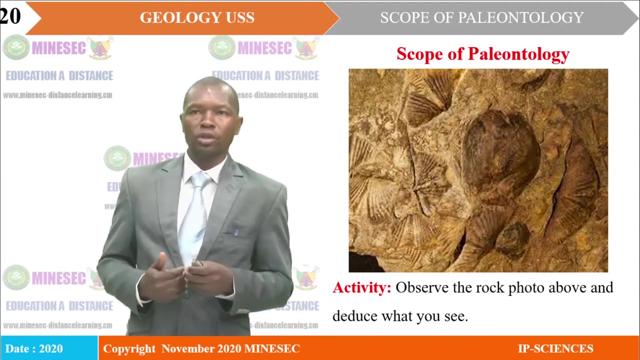 paleontology. now take a look at this photo. in the photo you shall observe and bring out the diagnostic elements as you observe. take note of the these impressions. these are fossil impressions on a rock body. now this guides us to the definition of paleontology, which begins the scope of paleontology. 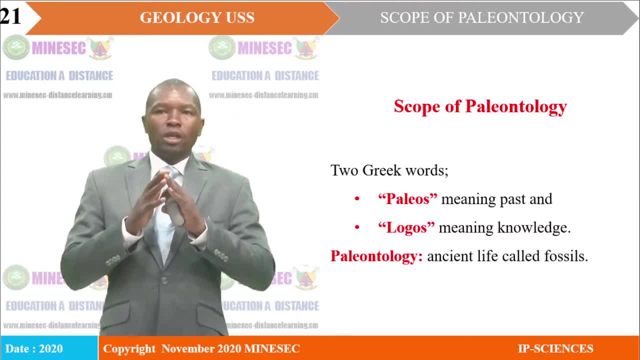 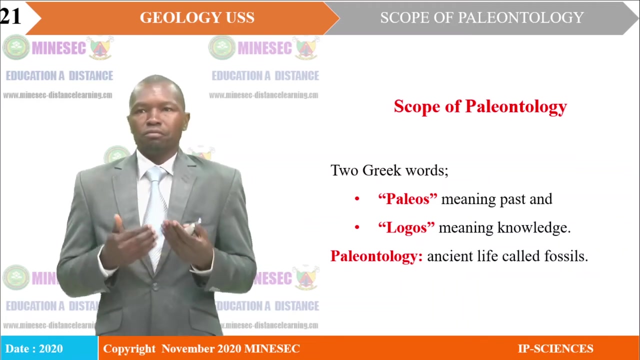 now, the term paleontology comes from two greek words. you have paleos, which means past, and then logos, which means knowledge. therefore, paleontology in its big sense is the study of ancient life, called fossils. ancient here captures past and then the past life. information that should be called fossils involves the knowledge that 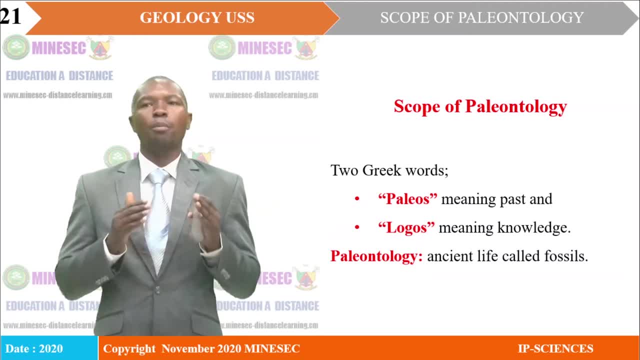 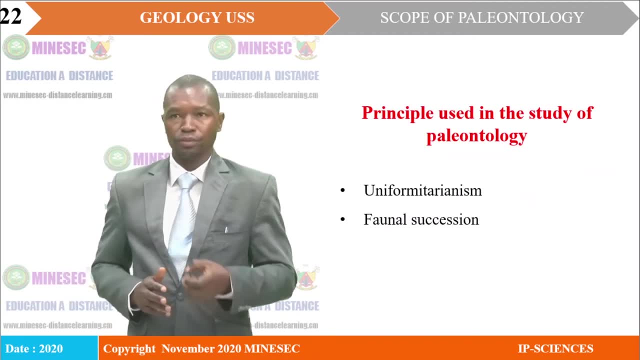 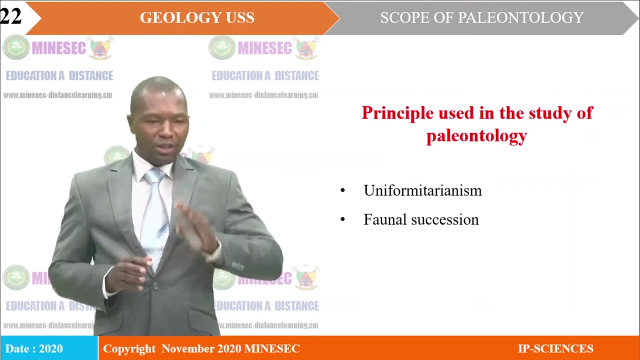 we are supposed to get. so, in general, paleontology is the study of ancient life, which is most likely called fossils. there are some principles that will guide the study of paleontology, the first of which is the principle of uniformitarianism. This principle holds that the present is the key to the past, which means that we 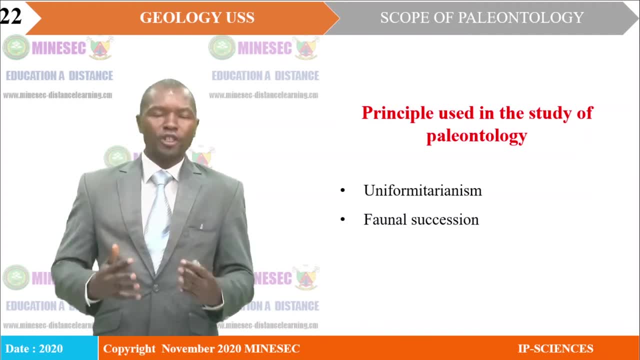 can look at the present way in which fossils are being preserved and we understand what happened with the preservation of fossils in the past. Again, we can look at the way organisms are living today and we try to judge on how they lived in the past. We also are so close and we hold so strong to the 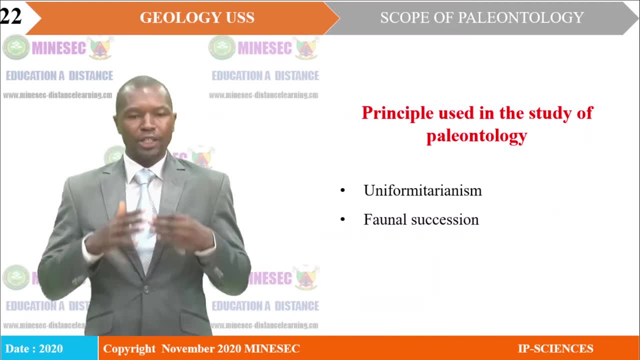 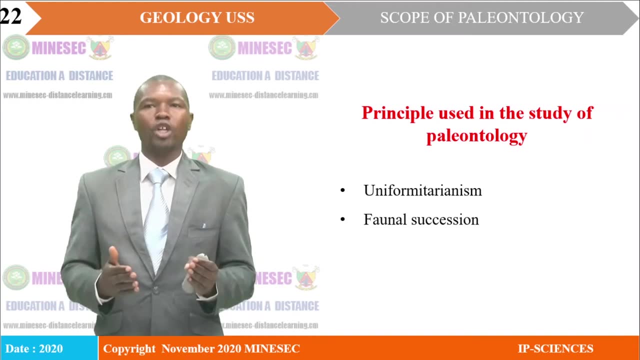 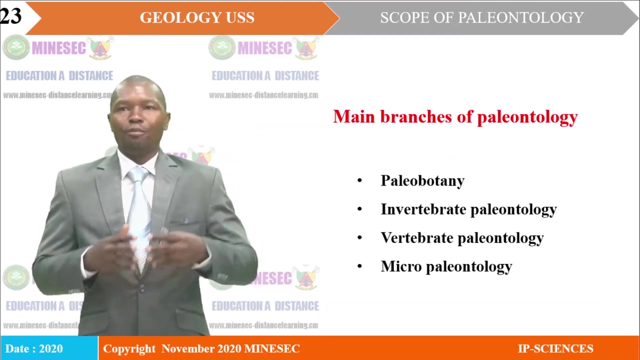 principle of fundamental association, which holds that if material is laid down in strata, and in each strata there are fossils, then it is possible to correlate the material based on their fossil record or to study each strata based on their fossil record. So the main branches of paleontology, We have paleobotany, we have invertebrate. 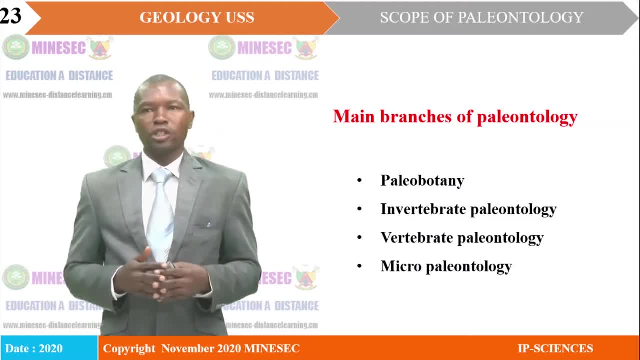 paleontology. we have vertebrate paleontology and we have micro-paleontology. Note should be taken here that we are using the British appellation, because in the American appellation paleontology is spelled using P-A-L-A-E-O-N-T-O-L-O-G-Y. 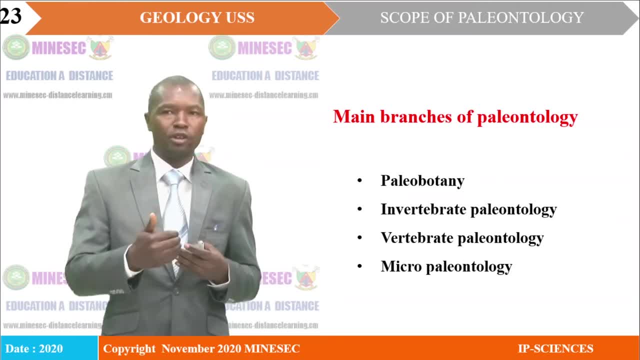 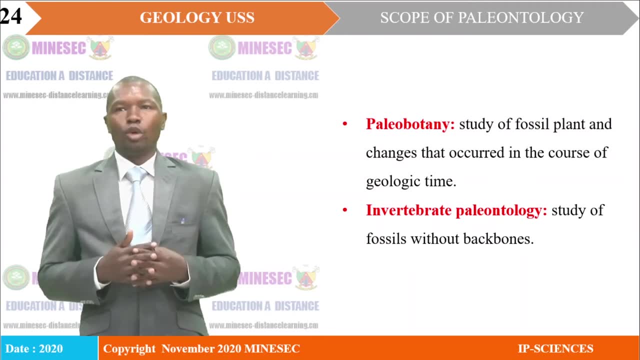 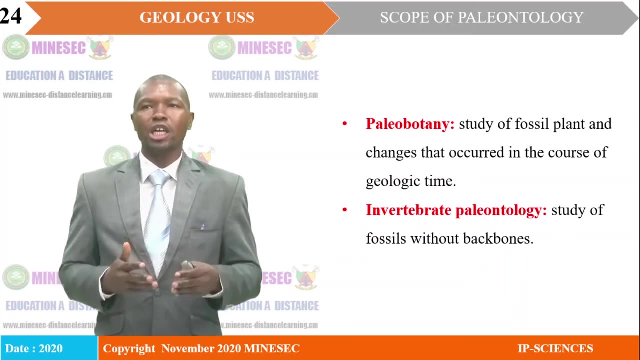 So the term we are using for paleontology is spelled in the British English. Then we begin with paleobotany. Paleobotany is the study of fossil plants and changes that occur within the course of paleobotany. Paleobotany is the study of fossil plants and changes that occur within the course of. 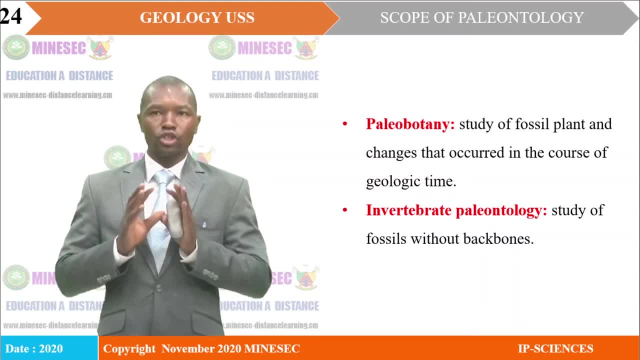 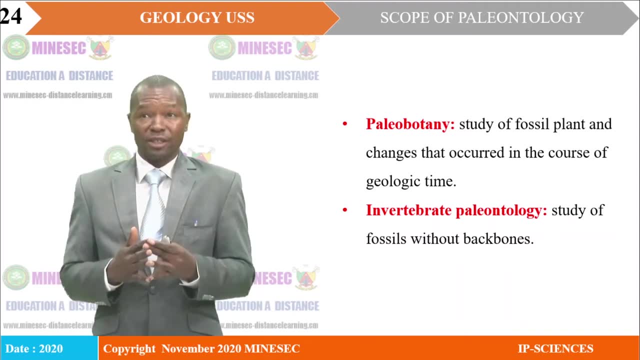 geologic time. So it has to do with paleontology that focuses on the preservation of fossil of plants, organism. Then we have invertebrate paleontology. This is a branch of paleontology that has to do with the study of fossils without backbones. So here we will focus attention with fossils without 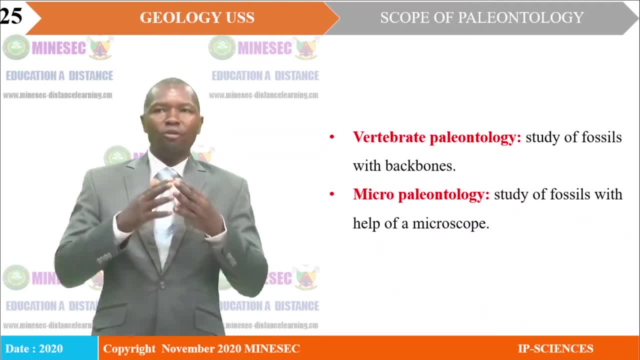 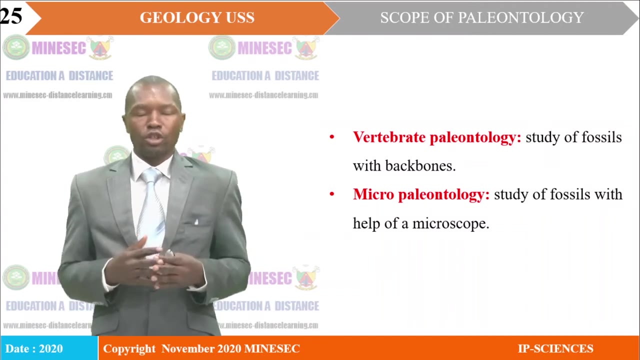 backbones. Then vertebrate paleontology is the branch of paleontology that deals with the study of fossils with backbones. We have mulocks, Then we have micro-paleontology. Just from the word micro, you have to know that it is. 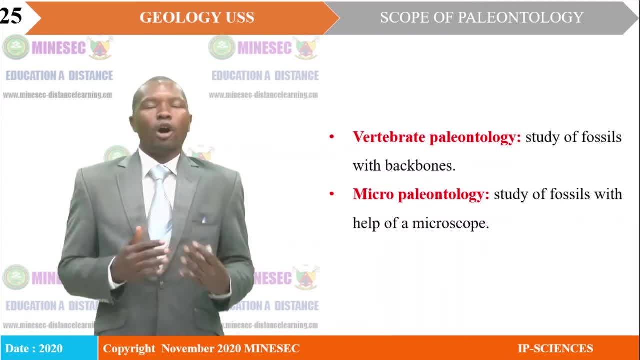 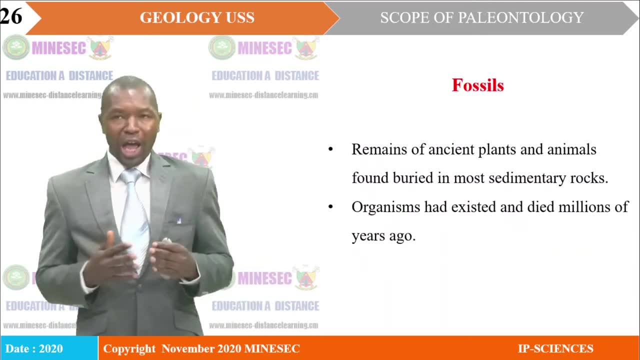 the study of fossils with the help of a microscope or fossil traces. This is the study of fossils with the help ofben Carson. the introduction to male coral, lightly important fossils. Now, now we will look at what a fossil is. In our phot investigations we saw some fossil impression, But what is it? that is a. 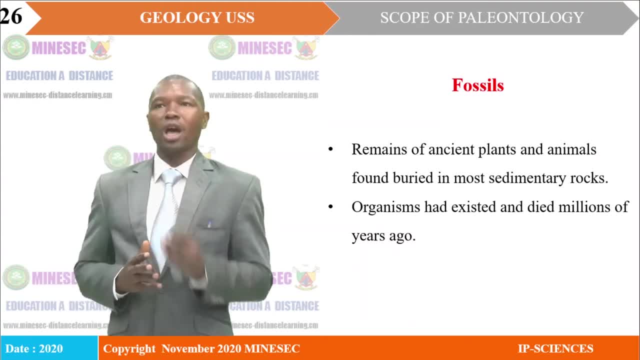 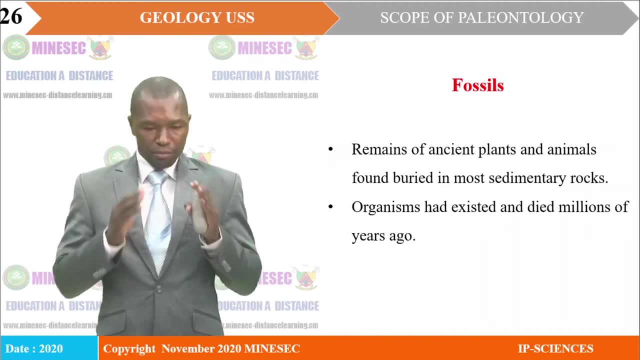 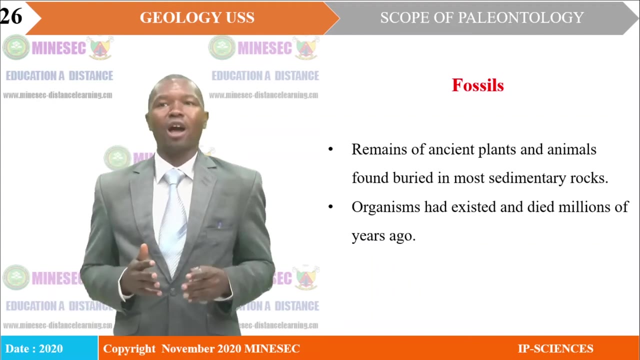 fossil, A fossil in geology or the fossils in geography, will involve the remains of ancient plants and animals found buried in most sedimentary rock. most underlined, most aavo sedimentary rocks will have fossils, but fossils are preserved in most sedimentary rocks organisms. 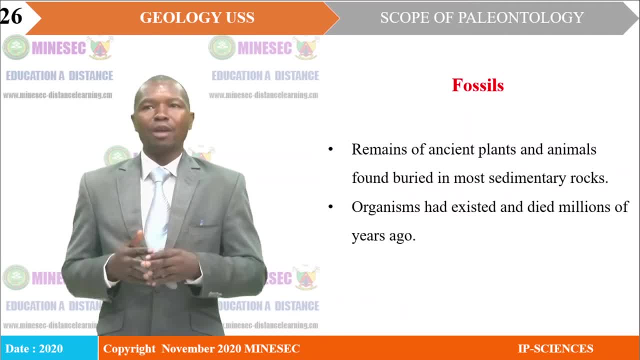 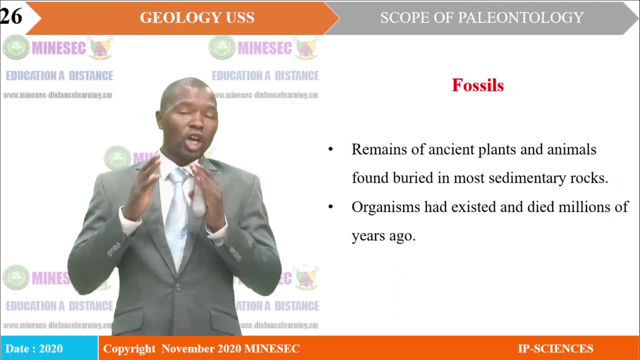 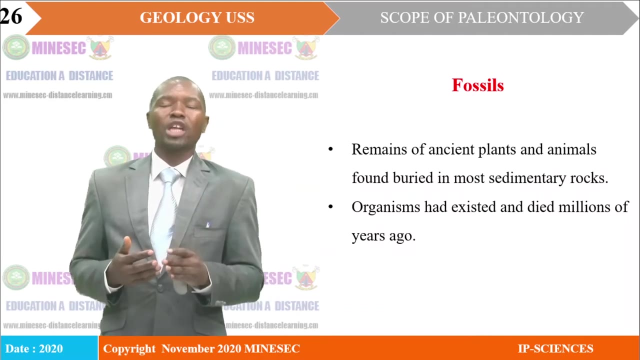 have parts or organisms have been exist, had existed and died millions of years ago. so when we talk fossils, we are not talking about material that is just organisms that are just preserved, present recently. we are talking about material that long lived and have been preserved, most especially in sedimentary rocks. 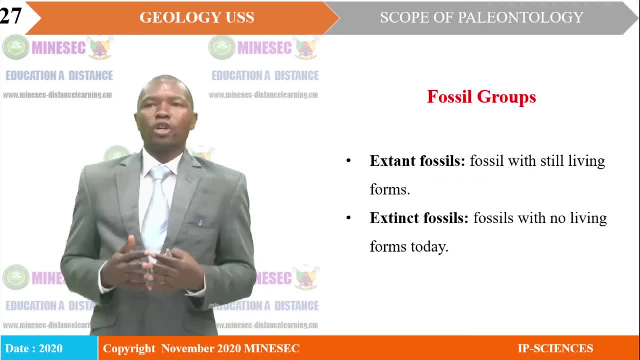 now fossil groups. the common fossil groups involve the external fossils and the extinct fossils. external fossils are fossils with still living forms. it means that there are fossils, that we still have their different forms present today, but we have some that lived in the past, where preserved in rocks, then in extinct fossils. we are talking about fossils with no living forms today. 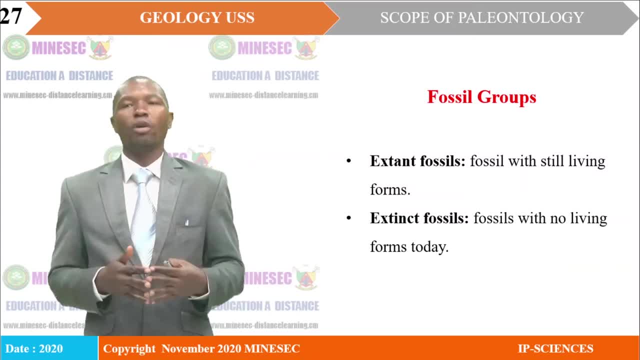 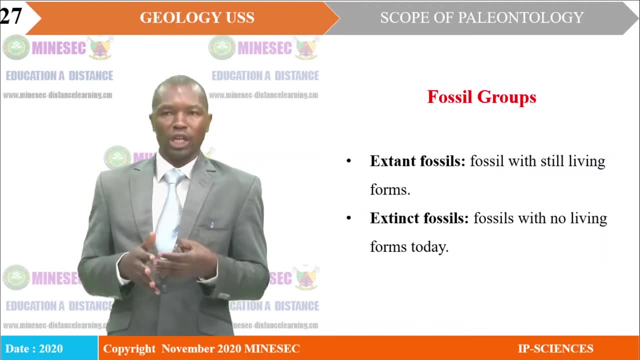 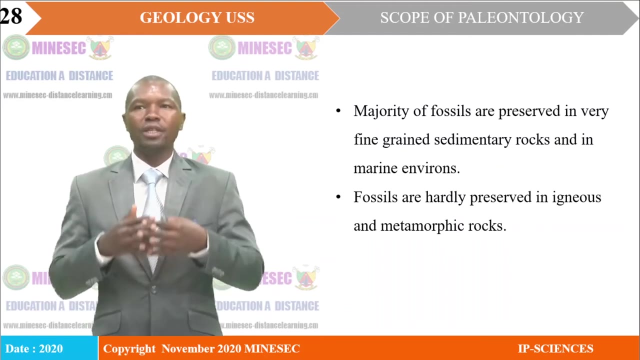 for example, you have the fossil trilobite. we don't have living forms today, for example, we have mollusks. we have mollusks that have been preserved, but we still have mollusks living. today. majority of fossils are preserved in very fine gray sedimentary rocks and in marine environments. 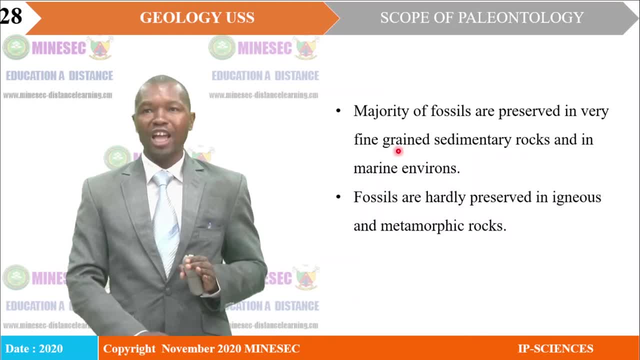 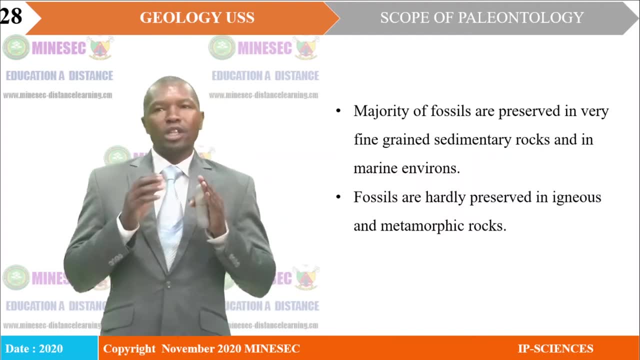 remember the key words. here you have fine grain, sedimentary rocks and marine environments. that is not to say that other environments may not have fossils or, better still, medium and coarse grain sedimentary rocks will not have fossils, but that they are most likely preserved in fine grain sedimentary rocks and in marine environments. fossils are. 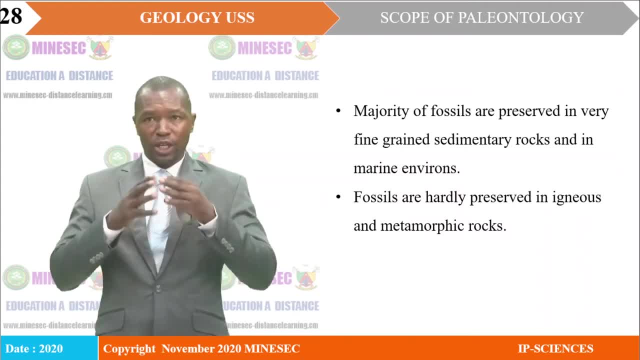 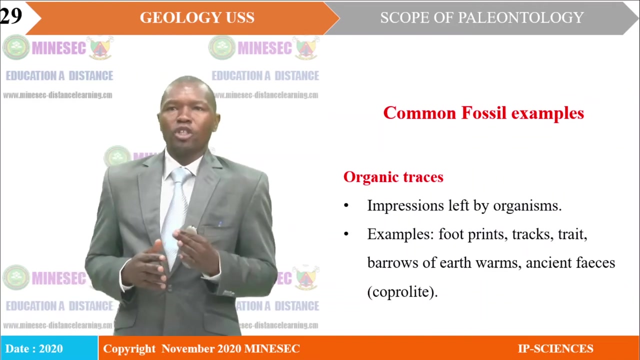 hardly preserved in igneous and metamorphic rocks. the reason is simple: these are rocks that are formed under harsh conditions of temperatures and pressure, and so the high conditions will most likely destroy the fossils. even if they were to contain the fossils now common fossil examples. the most likely common fossil examples include organic fossils. these are organic traces. these are: 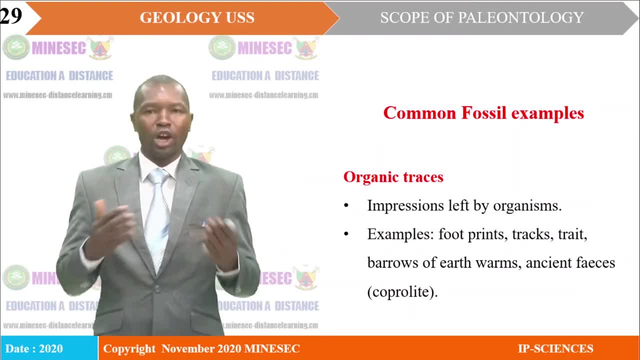 simply impressions left by organisms in a rock body. those impressions simply depicts that the organism had lived and then only allowed traces. examples will include footprints, you have tricks tracks, you have traits, you have burrows of egg worms and you have ancient physics which is most likely called coprolites. these are the common impressions that when you see in europe, it gives. 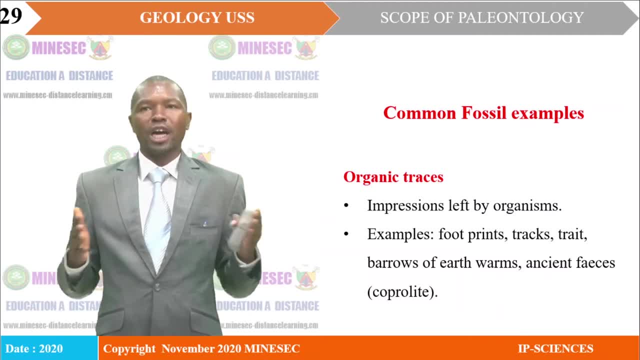 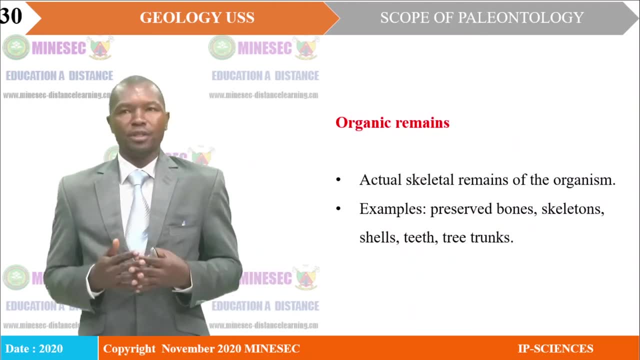 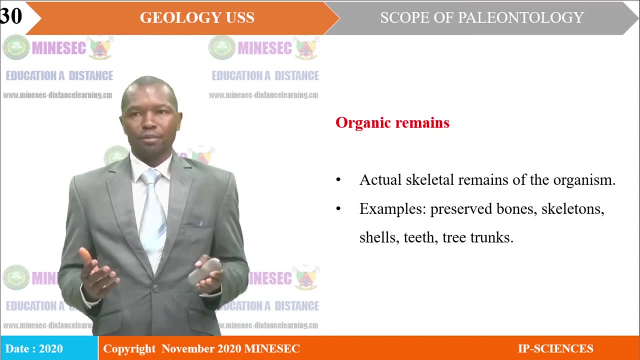 you the you gives you a practical example of an organic trace fossils. we have organic remains. this should be, uh uh, those actual skeletal remains of the organic remains of the fossil. we have organic remains. this should be, uh uh, those actual skeletal remains of of the organic remains of the fossil. we have organic remains of the organisms that had lived in the past. 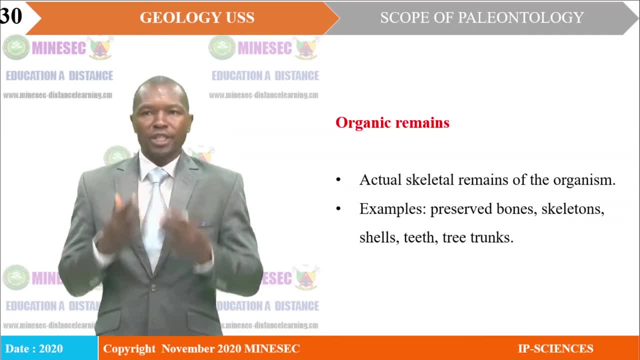 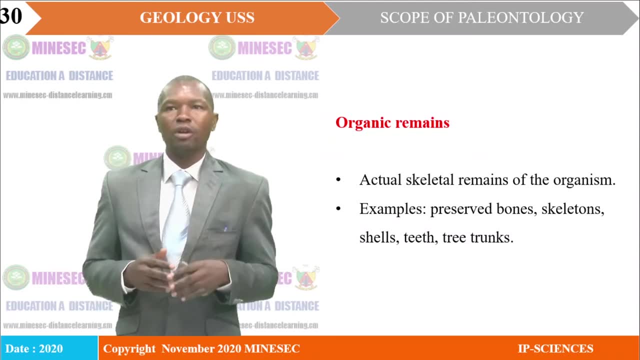 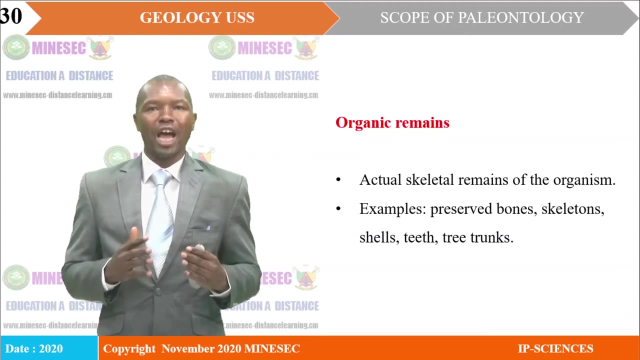 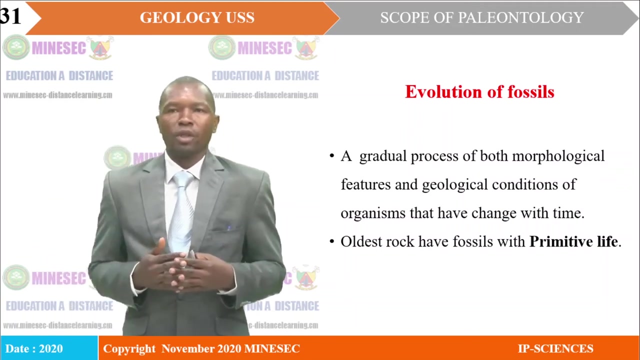 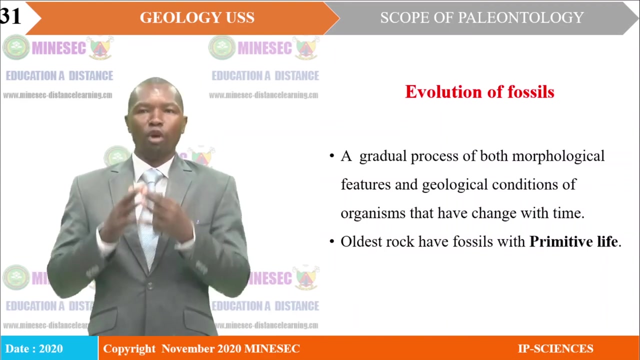 of the organisms that had lived in the past and were preserved in rocks. examples will include preserved bones, skeletons, shells, teeth and tritons. those are organic remains that you have most likely preserved as fossils. evolution of fossils: here we are talking about the gradual process of both morphological features and 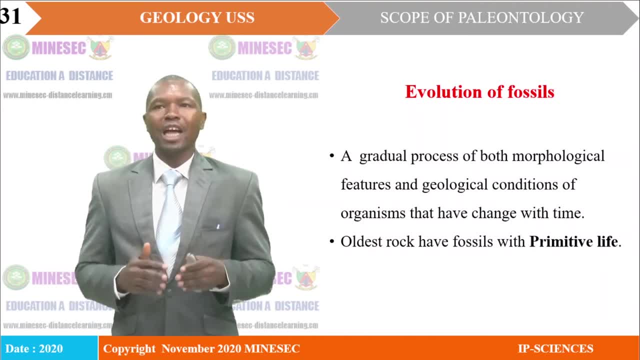 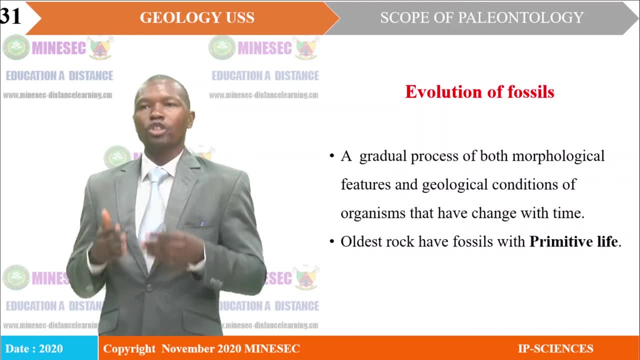 geological conditions of organisms that have changed with time, from the most primitive to now the most simple forms. so fossil evolution will involve key things: gradual process and geological conditions. and geological conditions. remember that soon we will look at conditions necessary for fossilization. so in evolution we must take note of the different morphological features, that is, the different features that are: 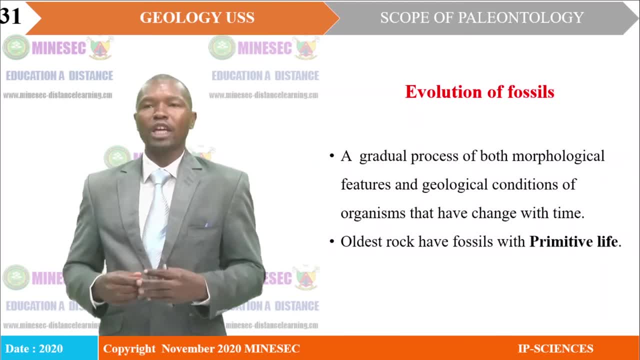 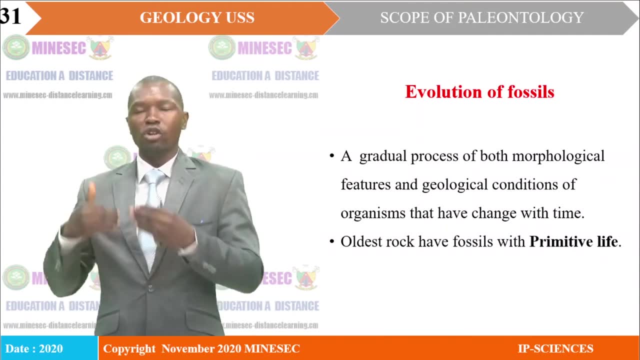 visible features that we can observe, that we can demonstrate and that we can measure within a fossil organism in order to give it the normal evolution we can observe in the fossil organism. uh, how are full descriptive, a full description. so all the rocks, or the oldest rock, will have fossils? that 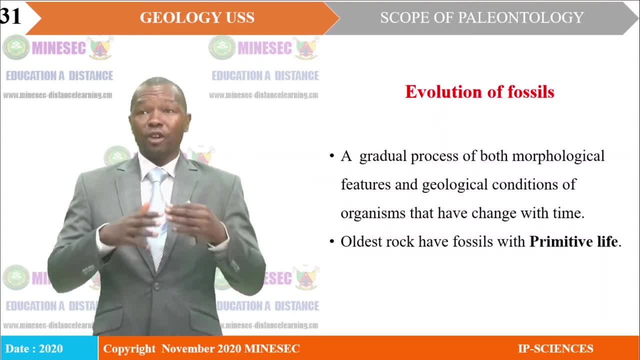 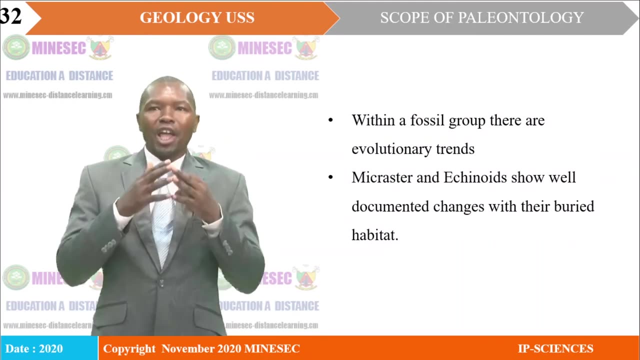 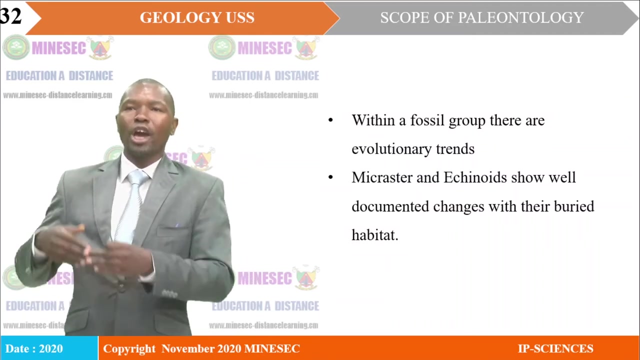 are that have a primitive kind of life. so the more older fossils are, the more primitive they will be, also within a fossil group. there are evolution- our trades- and this evolution- our trains- tells the story of how the organism had lived and which conditions permitted it. for example, you have my class. that are egg notes. we show well documented changes within their buried. 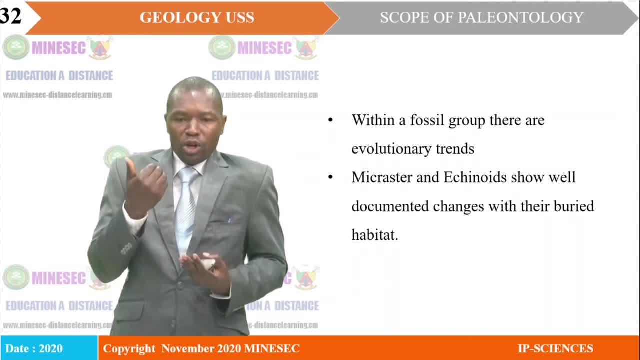 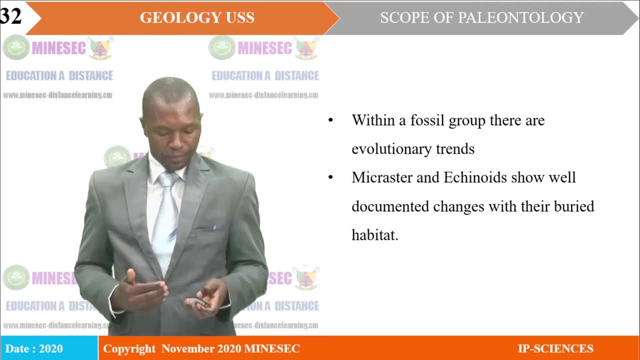 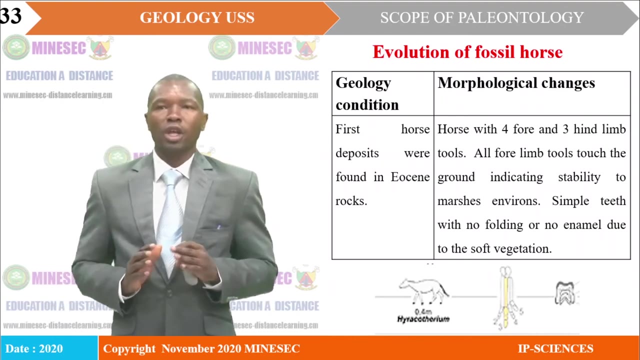 habitats. so when you see those impressions, it will give you a picture of how the organism was living, the conditions under which it lived. now we'll take the case study of the evolution of fossil halls. now we are going to tabulate it. on one side we have the geologic condition and the other side will have the morphological. 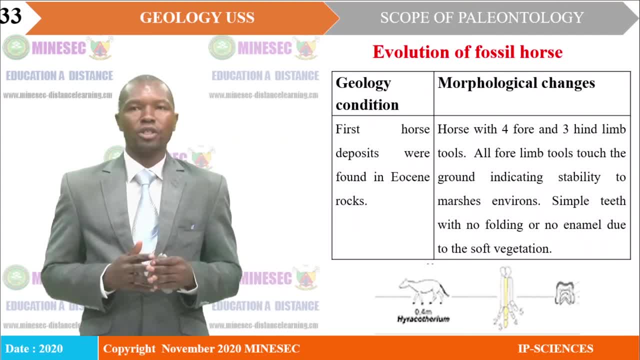 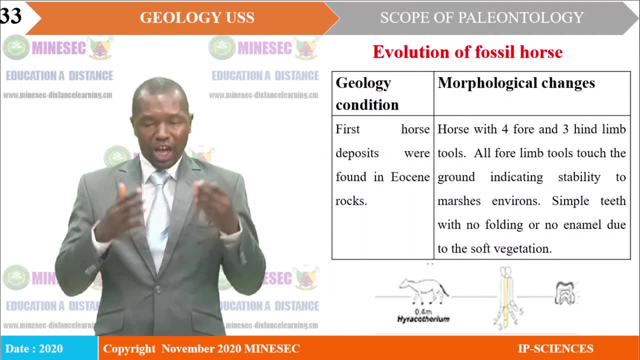 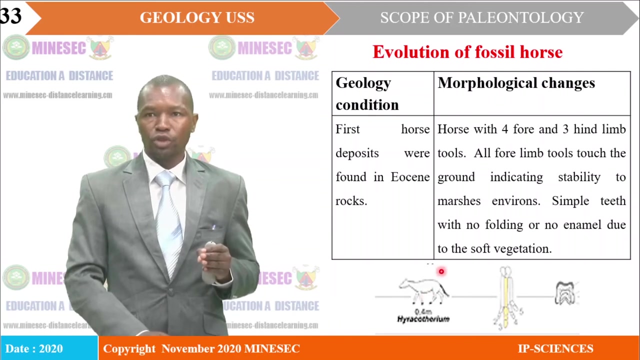 changes. now we have the first horse we deposit with deposit which was deposited in aoc rocks or which are found or preserved in aoc rocks. this horse had, uh had four, uh four and three high limbs, uh, high limb tools, and all the limb tools touch the ground, as you can see in this photo. 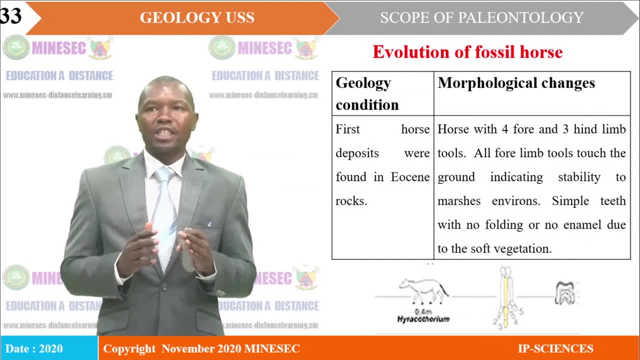 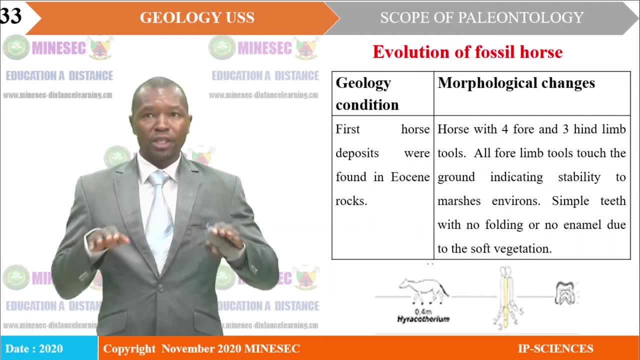 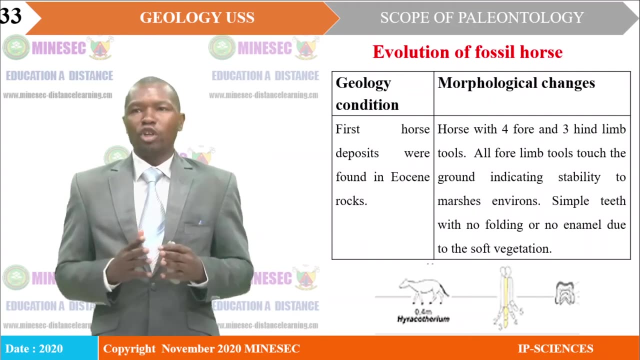 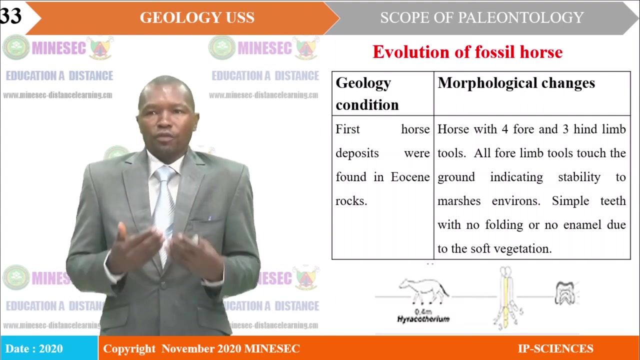 now essentially is the fact that they they. this indicates the conditions under which they lived, meaning that the conditions were machine. then again they have a simple teeth with more, with no folding or no external external teeth due to the fact that they had lived on soft vegetation, as you can see in this, in the 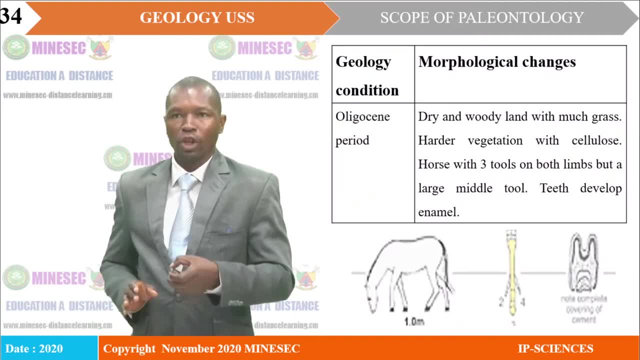 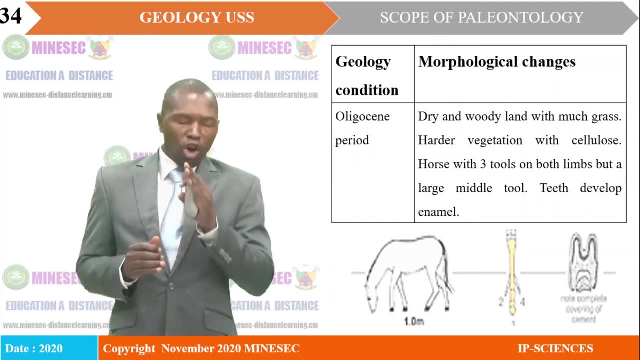 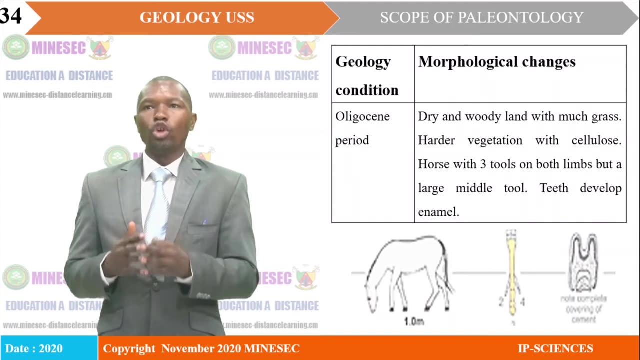 diagram that is provided. The second case is the Oligocene period horse. Now, the common morphological changes in the fossil horse were the fact that it has dry and woody land with much grass, indicating how strong that horse would have developed its teeth. So the 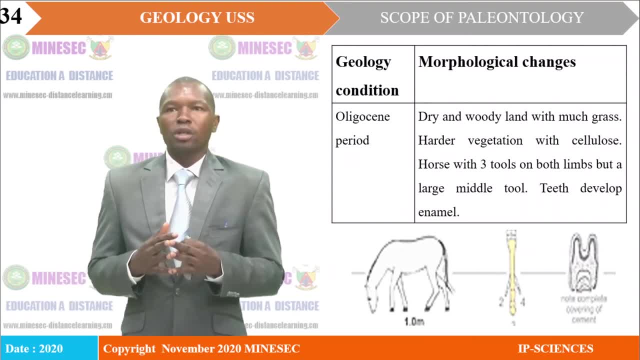 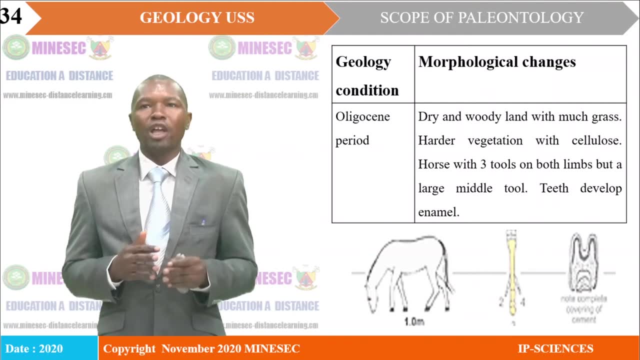 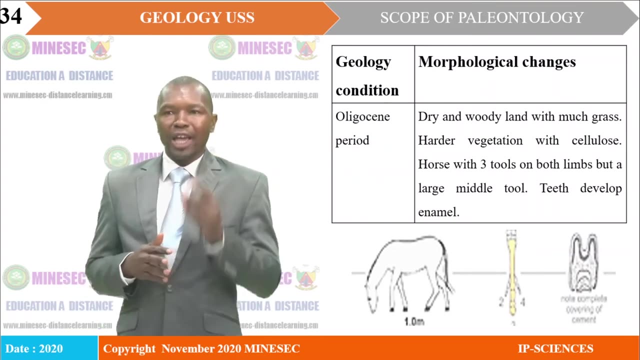 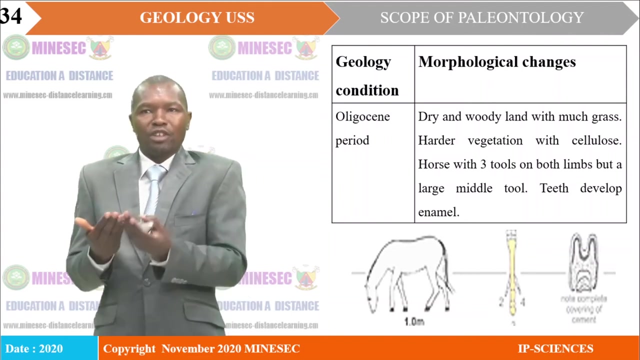 harder vegetation with cellulose will now depict a horse with three toes on both limbs, but with a large middle toe. The teeth develop enema. Enema here already tells us that the conditions were too dry and woody. Therefore it would have lived on very hard vegetation. 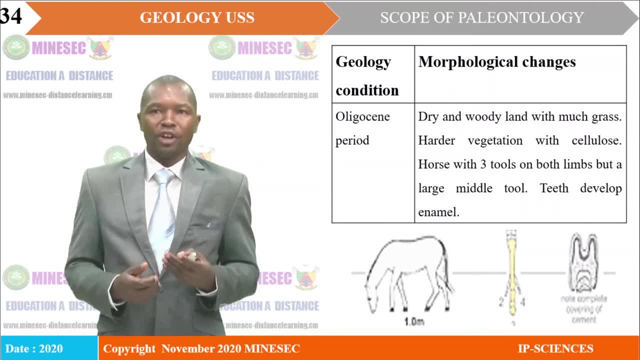 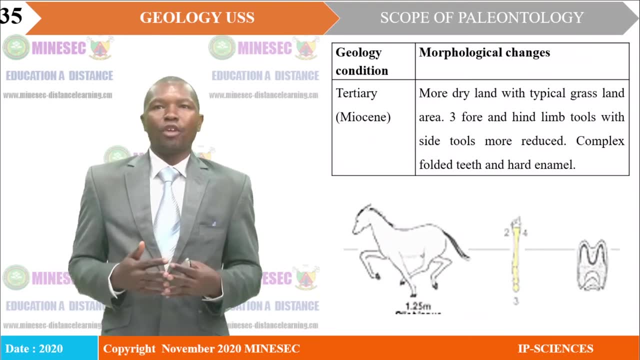 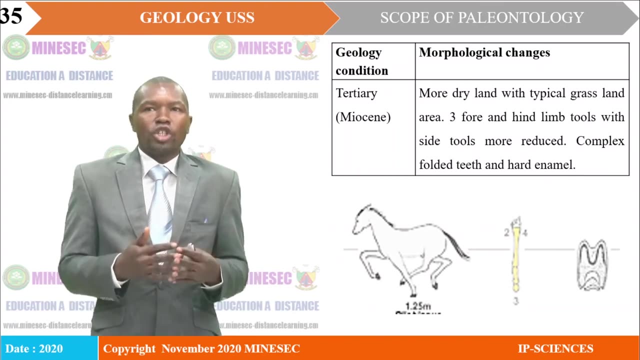 So it requires a hard enema, well-developed. Then you have the tertiary or the myocene horse. Here the conditions are more dry and typically grassland, with three, four and high limbs, limb toes on either side of their toes. 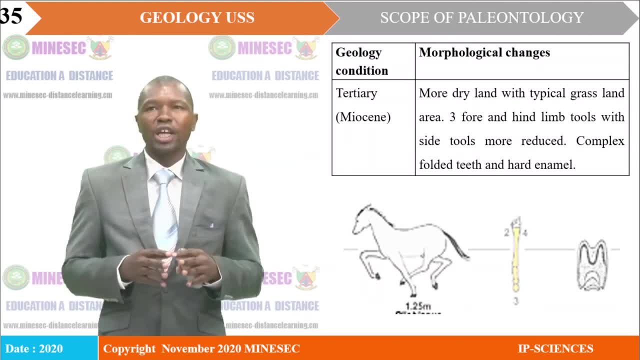 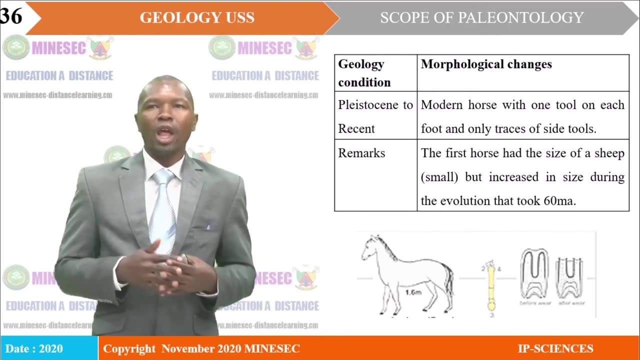 but this time around more reduced. Then they have complex folded teeth and hard enema, showing that the conditions are becoming more and more hard and it needs a hard enema to be able to crush its foot. Then you have the Pleistocene and, of course, the most recent horse. This is a modern horse. 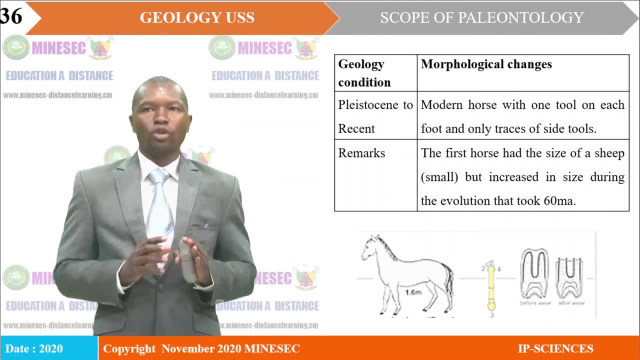 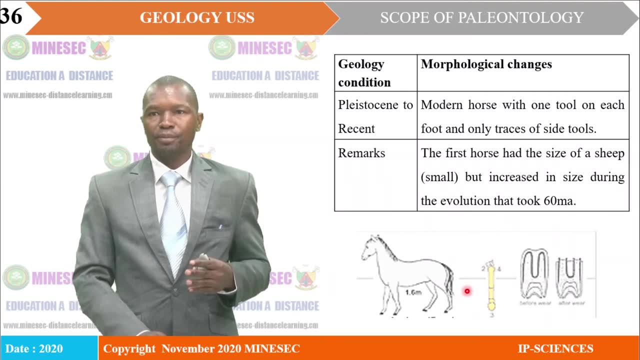 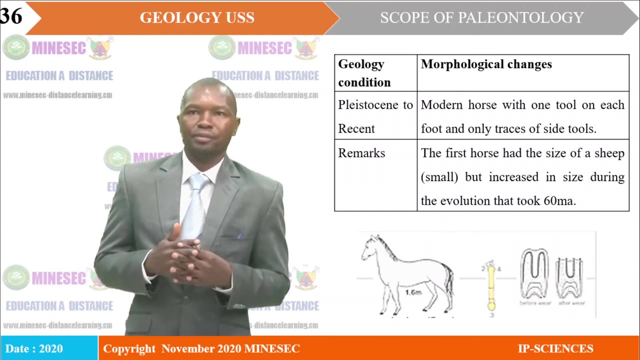 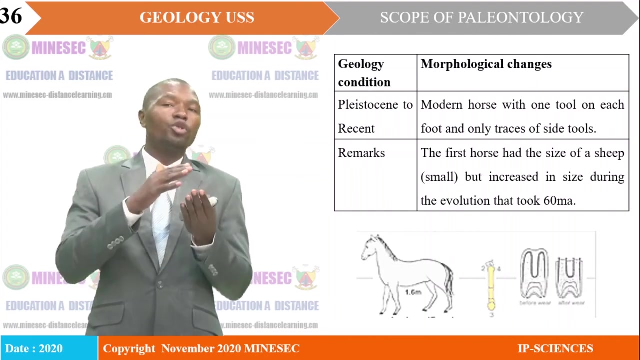 with one toe on each foot and the only traces of side toes You can see in the diagram. Now the teeth here should have very strong enema. That is the horse we see. now, When we talk about most recent conditions, we are talking up to when. 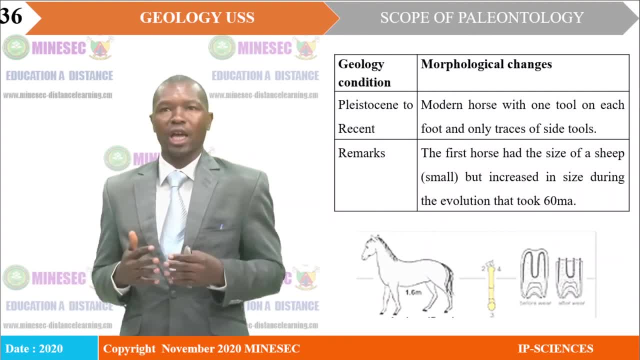 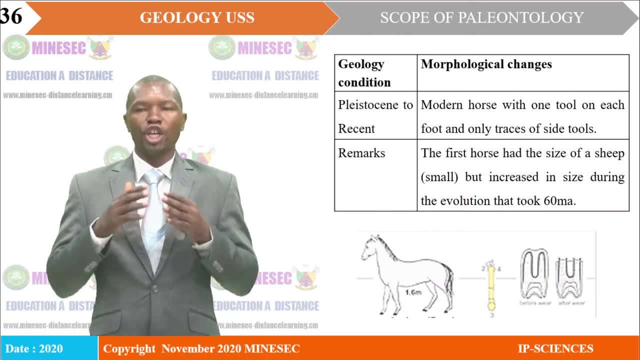 the evolutionary trait has been measured within the geologic time scale. Then to remark is the fact that the first horse had the size of a sheep. That is very small Then. the is very small then, but as it increased in size during the evolution, that took, uh, that gave. now. 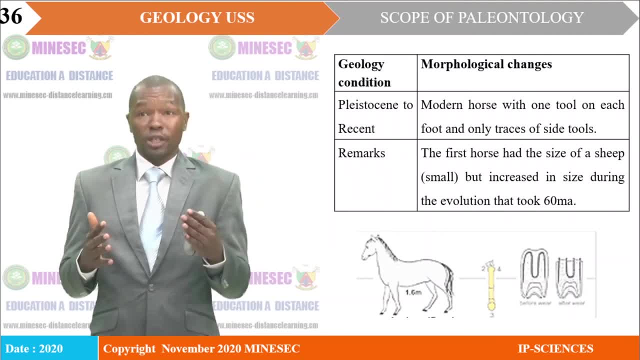 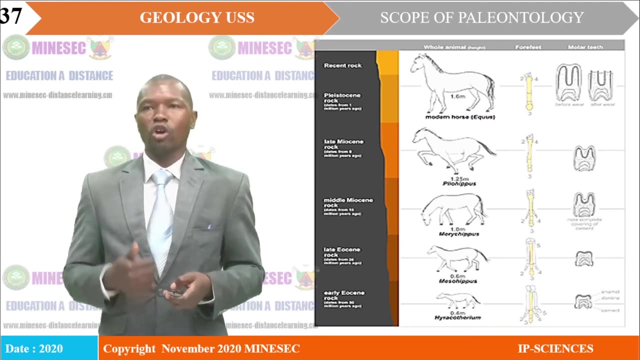 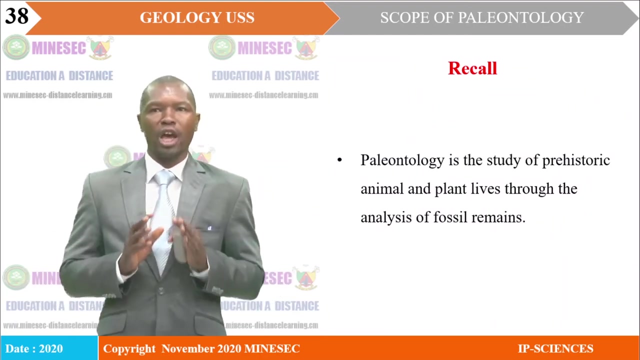 a size of a horse, of about the present size, which is bigger than the initial horse. that evolutionary train had gone through 60 million years. that is the practical picture of how the evolutionary train follows now. recall that paleontology is the study of prehistoric animal and plant lives through the analysis of fossil remains. easily put, it is the study of ancient life. 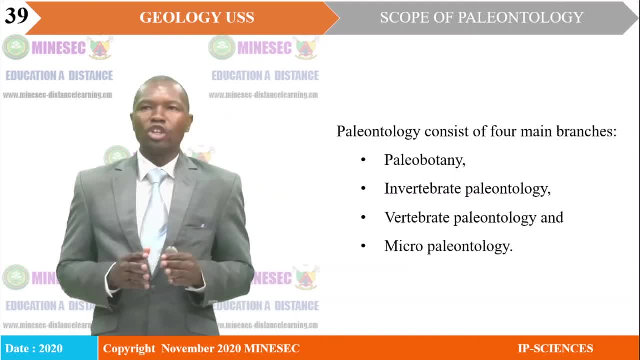 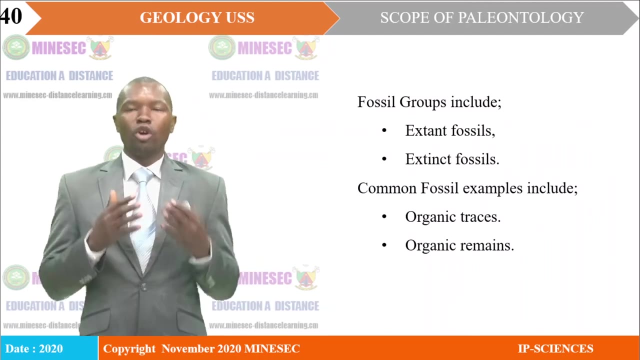 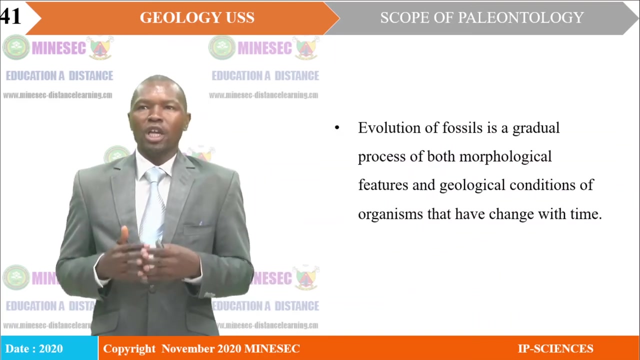 called fossils. paleontology consists of four main branches. you have paleo botany, invertebrate paleontology, vertebrate paleontology and micro paleontology. fossil groups will most likely include external fossils and extinct fossils. the common fossil examples include organic traces and organic remains. evolution of fossils is a gradual process. 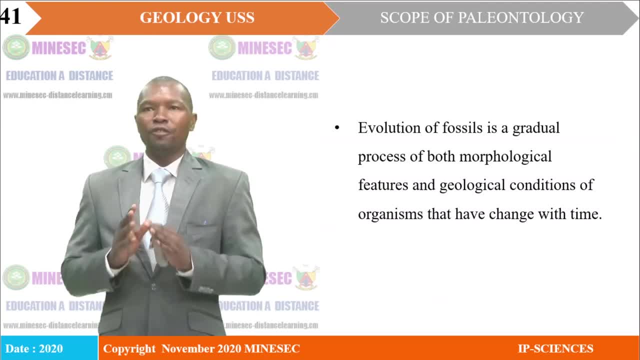 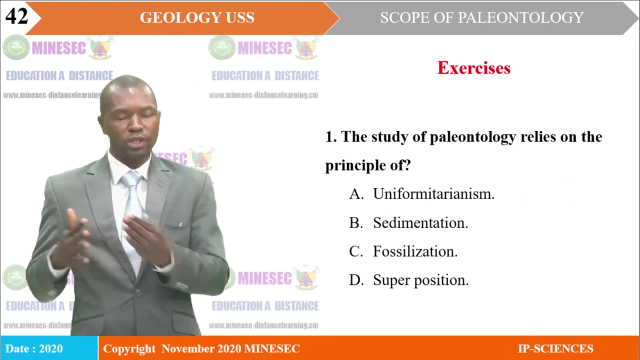 of both morphological features and the geological conditions of organisms that have changed with time. remember that time here should be in terms of time of millions of years, like the case of the frozen horse that we saw it going through an evolutionary trade of 60 million years. 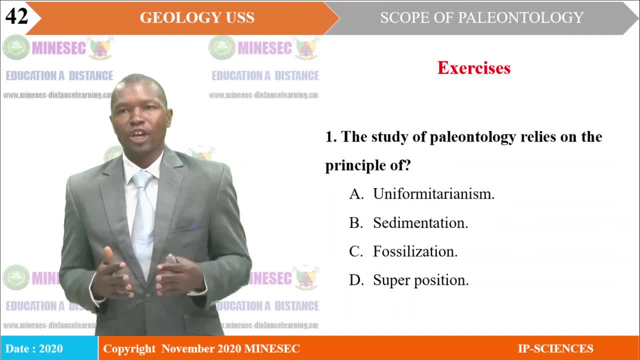 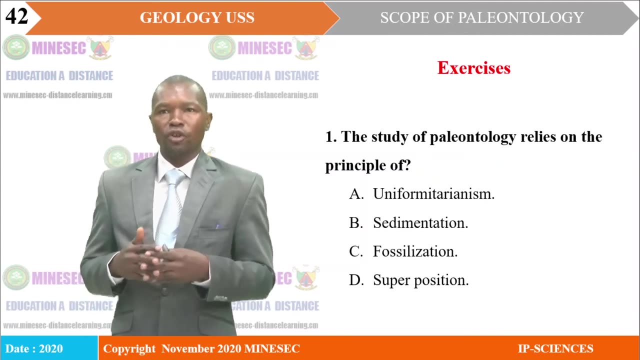 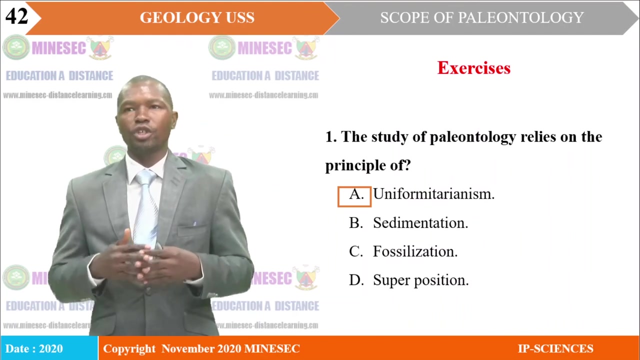 We shall now move into our exercises. The first one is: the study of paleontology relies on the principle of: A- uniformity and neonism, B- sedimentation, C- fossilization, D- superposition. Our correct answer is: A. the study of paleontology relies on the principle of uniformity and 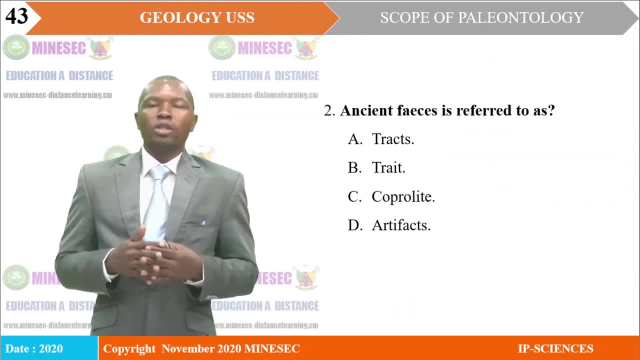 neonism. The second ancient physiques is referred to as A traits, tracts, B traits, C, coprolites, D- artifacts. The correct answer is C. ancient physiques is referred to as coprolites. 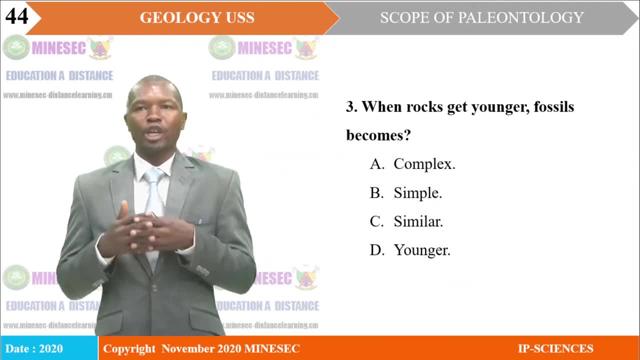 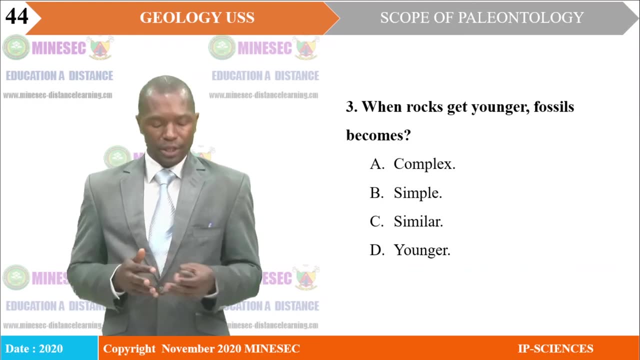 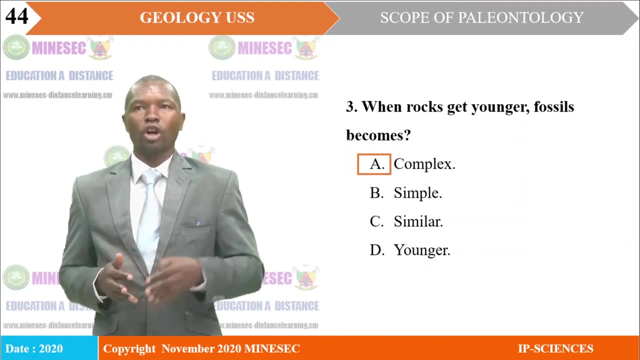 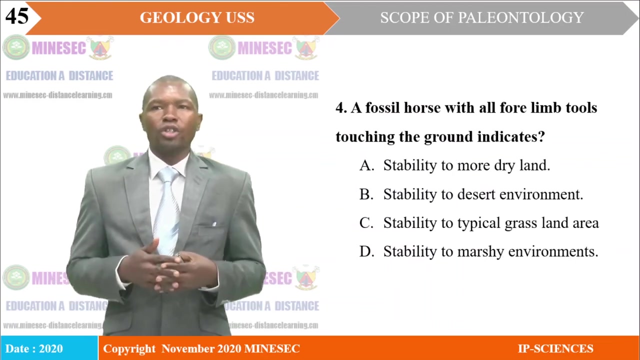 When rocks get younger, fossils become: A. complex, B simple, C. similar, D- younger. The correct answer is A. when rocks get younger, fossils become more complex because older rocks will contain primitive fossils. Next, A fossil horse with all four falling toes touching the ground indicates A stability. 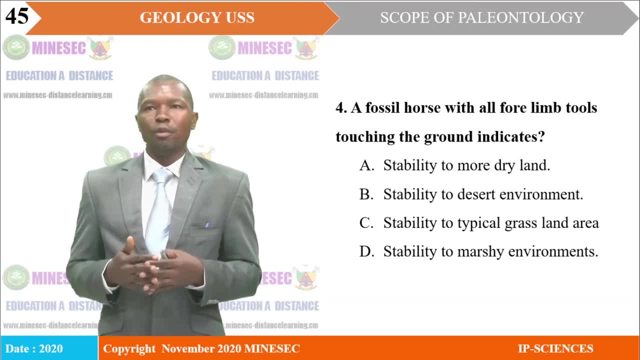 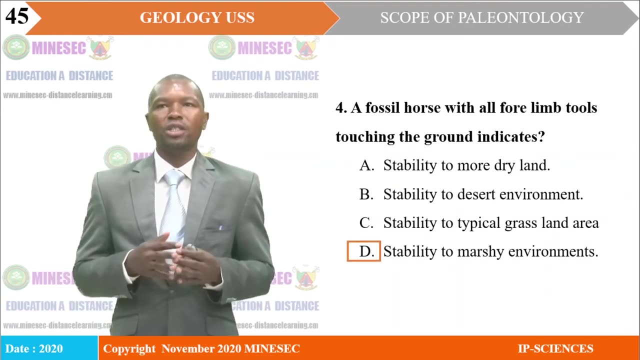 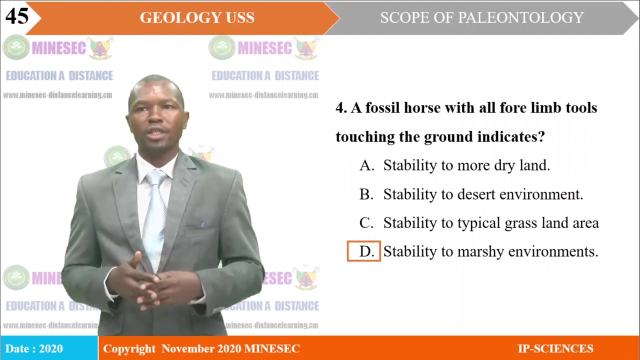 to more dry land. B- stability to desert environment. C- stability to typical grassland area. D- stability to marshy environment. Our correct answer is D- a fossil horse with all four falling toes touching the ground. Next, A fossil horse with all four falling toes touching the ground indicates A stability to marshy.